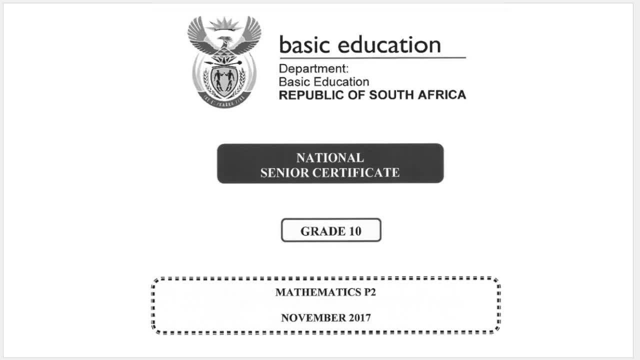 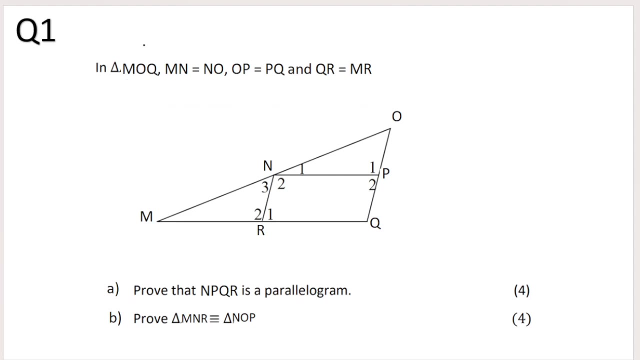 a few basics, a few things that you must know in order to get full marks for these questions. So make sure that you're taking down notes. Let's get into question number one. My first question says: in triangle, MOQ. they tell me MO equals O, OP is equal to PQ. 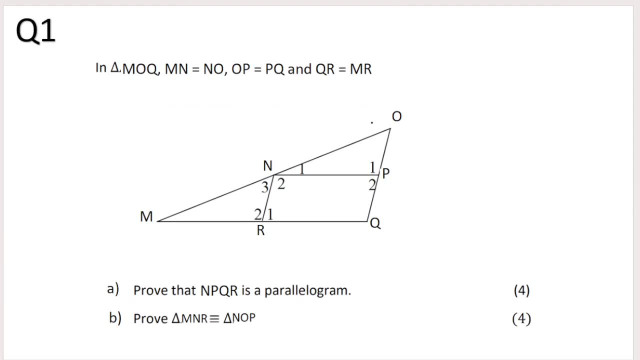 and QR is equal to MR. Now, first of all, when it comes to Euclidean geometry, you're always given a little written piece of information and you're given a diagram. There is, and there always will be, information indicated on the diagram, but sometimes not all of the information that is included in the paragraph. 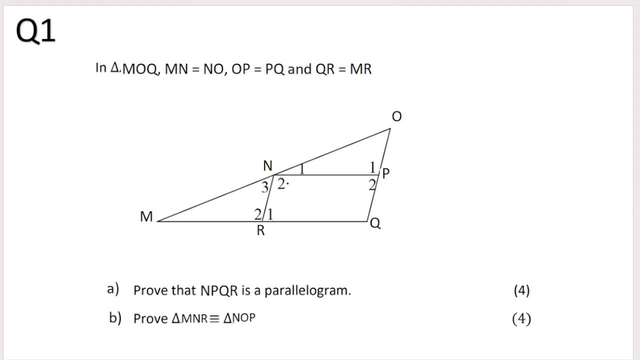 above or before the diagram is included on the diagram itself. So always make sure that you fill out all the information on the diagram that's mentioned in writing but is not necessarily put on the diagram. So it says MN is equal to NO. So that tells me that this length over here is equal to this length over here. They also tell me: 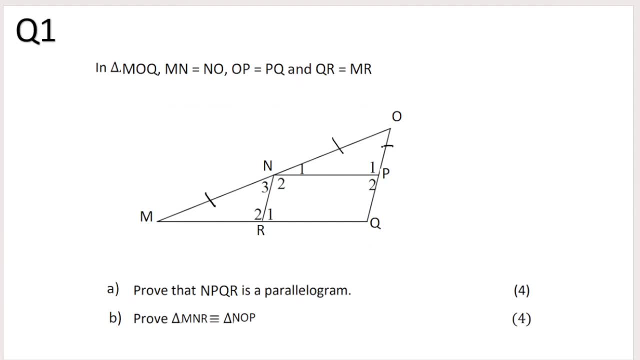 that OP is equal to PQ. So OP is this length over here and it's equal to PQ, which is this length over here. And then they say QR is equal to MR. So QR is this one over here at the bottom. They say it's equal to MR. So they give me a whole bunch of sides that equal one another And my. 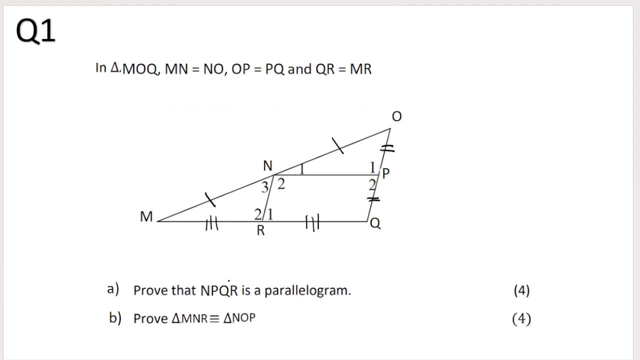 first question says: prove that NPQR is a parallel. Now, first of all, we have a big triangle, We have smaller triangles and we have a parallelogram. Let's just highlight the parallelograms so we can see what we working with in PQR. that is over. 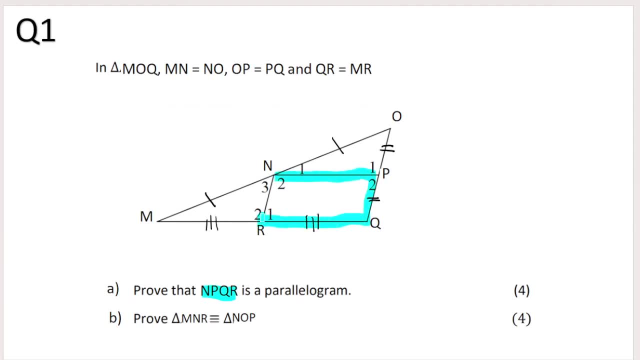 here. So they want me to prove that. this over here is a parallelogram. First of all, let's just make sure that we have all the information included on my diagram now. Yes, I do. We don't have the size of any angles. We have nothing else like that. They've just labeled some of the singles. 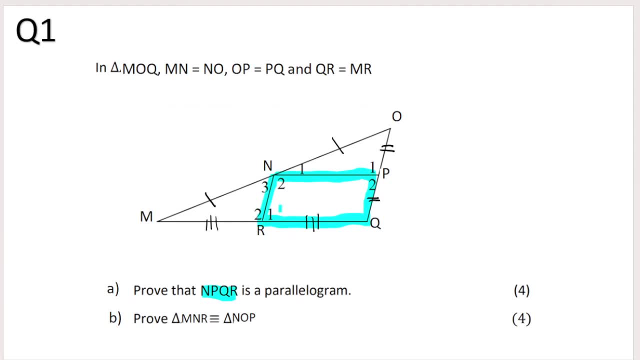 that, for example, this angle over here is called angle r1, this one over here is called angle r2. we may make use of that later, especially when we are proving congruency in question 1b. but let's tackle the first question, and that is proving that npqr is a parallelogram. so the first thing that 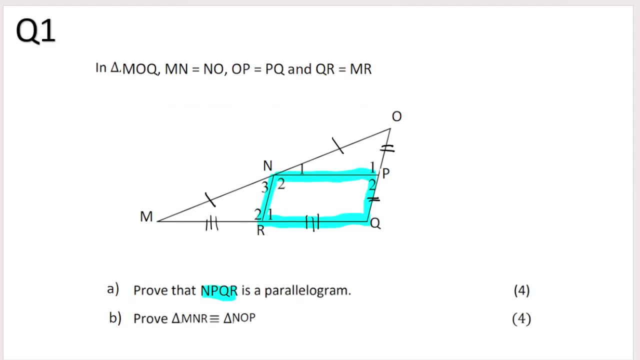 you need to know when you see a question asking you to prove that a quad is a parallelogram, is you need to remember how can i prove that a quadrilateral is a parallelogram? what criteria do i have to show? what criteria do does this quad have to meet in order for it to be a parallelogram? 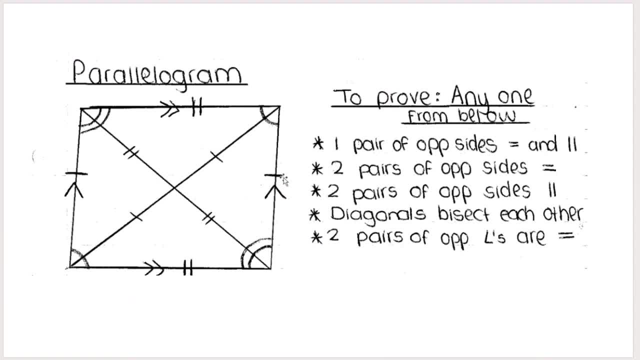 or be classified as a parallelogram. so this comes from my summary, which basically summarizes the things that we need to do. in order to prove that a quadrilateral, so a shape with four sides- is a parallelogram, you need to prove one of the following things. 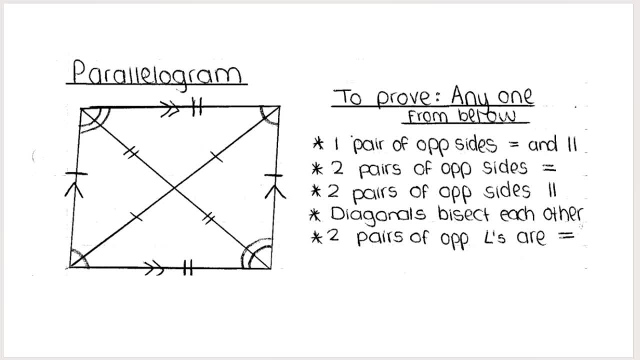 so either you need to tell me that both, that one pair of opposite sides is equal and parallel, so one pair of opposite sides both equal and parallel, or you can show me that two pairs of opposite sides are equal or two pairs of opposite sides are parallel, or that the diagonals bisect. 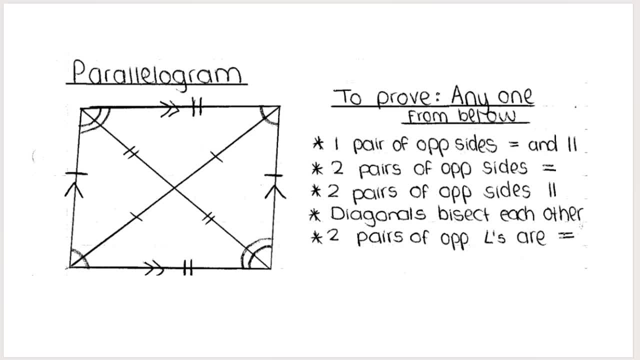 each other or that two pairs of opposite angles are equal. now we have to think, in terms of the context of our question, which one of these makes the most sense to prove that a quadrilateral is a parallelogram. now if we go back to the question, you'll see that we don't have diagonals in the question. 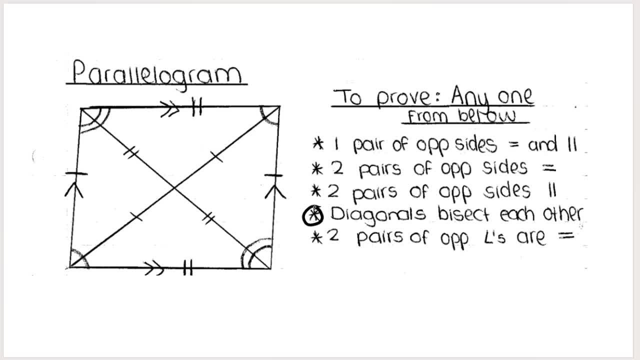 so we can't use this to prove that it's a parallelogram. we also can't use the angles, because we're not given the values for any angles in that question, so we can't use this one. so we're either going to have to prove two pairs of opposite sides are equal or two pairs of 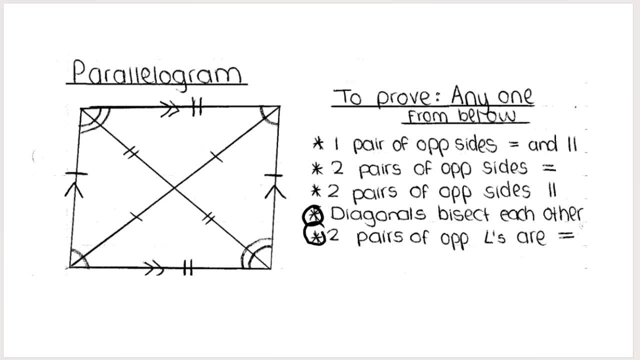 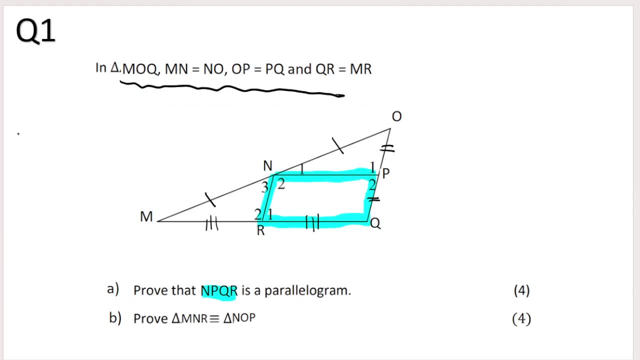 opposite sides are parallel. so let's go back to our diagram and i'll show you what i mean now. remember, they gave us all this information in the beginning of the question for a reason. now they're telling me mn is equal to no, so we know that this. 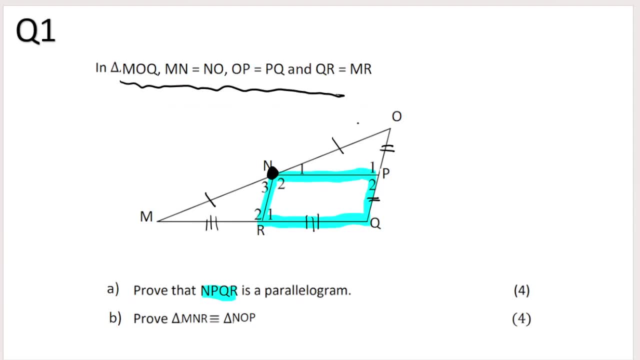 n is the midpoint of line mo. they also tell me that op is equal to pq. op is equal to pq, so p is the midpoint of that line and qr is equal to mr. qr is equal to mr, so we know r is the midpoint of that line. now, now i hope you're thinking in the correct way, or in the right direction, and 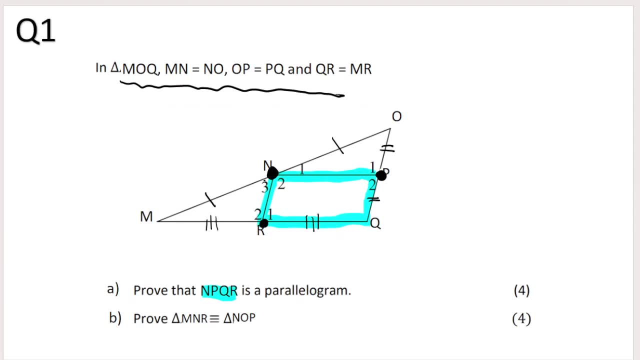 if they're telling me that this line is equal to that line and therefore we have the midpoint, we have the midpoint there, we have the midpoint there. we actually have three midpoints. i hope that you can see that we may use midpoint theorem in order to get towards our answer. so i'm going to break. 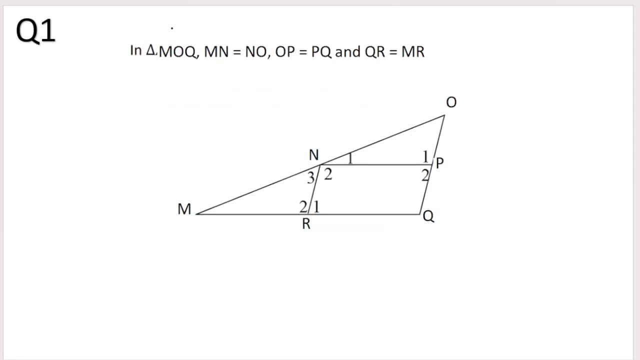 it down a little bit um slower for you. if i say mn is equal to no, okay, so we said that's equal to that. that's making n the midpoint over there, and op is equal to pq. so that is that. one is equal to that one. now we have the midpoint over there as well. 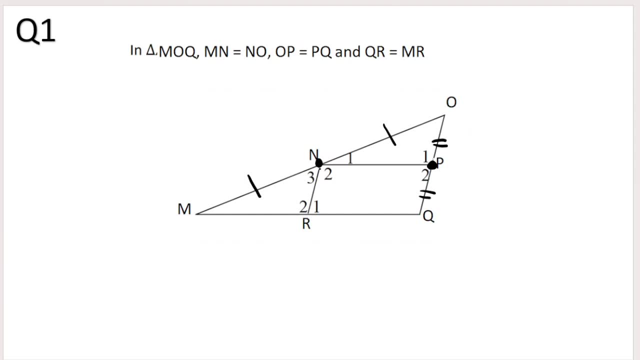 so we see we have n being the midpoint of that line, m, o and p being the midpoint of this line, oq. and what do you know about the midpoint theorem? if i draw a line connecting those midpoints over there, i know that that line is parallel to this line. you should remember the midpoint theorem. if you don't, 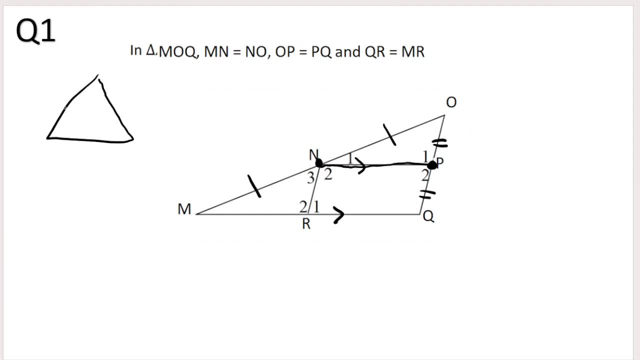 i'll link a video of mine in the description about in the above or in the description below. so if you have two midpoints like that and you join it with a line, it means that that line joining the two midpoints is parallel to this line over here. so so far we know that np, this line over here, np, is parallel to this line over here. 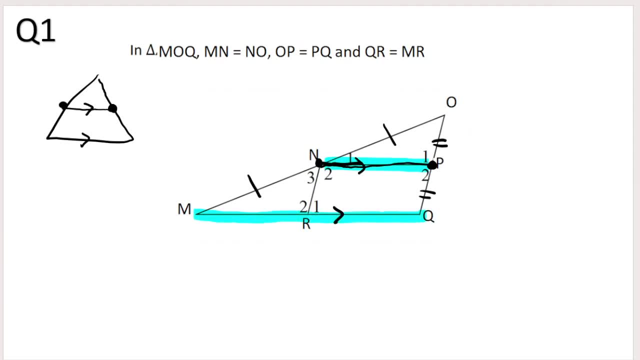 mq. and why is that helpful? remember, in order to prove that a quad is a parallelogram, we can prove two pairs of opposite sides are parallel, and we have now just proven that np is parallel to rq or mq. okay, so we're almost there. now we just need to somehow prove that these lines over here are also parallel. so let's just write out: 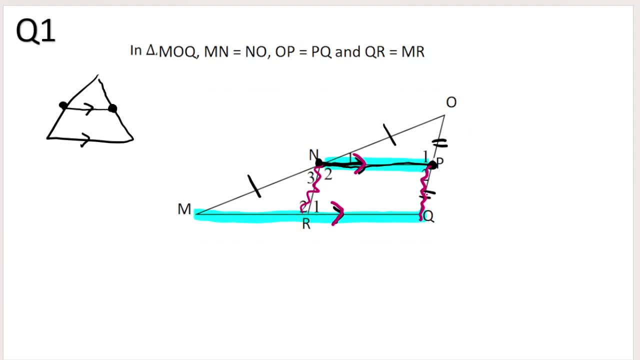 what we've just proven. that let's with a statement and a reason. in euclidean it's always statement and reason. So, using the midpoint theorem, because they gave me n as being the midpoint of that line and p as being the midpoint of that line, I can therefore conclude: because of the midpoint, 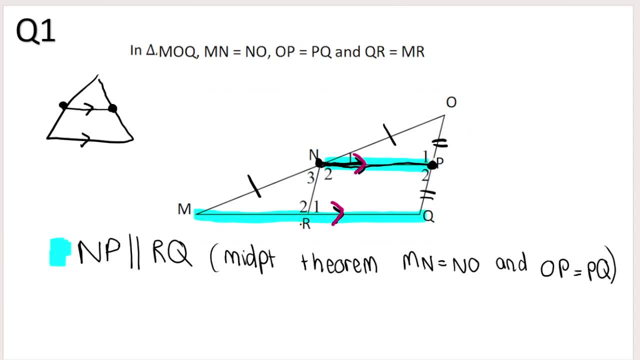 theorem that np is parallel to rq. okay, Parallel to mq, but r is on the same straight line, so rq, So np parallel to rq. that's our first pair of opposite sides being parallel. that we've now proven. So we are halfway to proving that that shape is in fact a parallelogram. 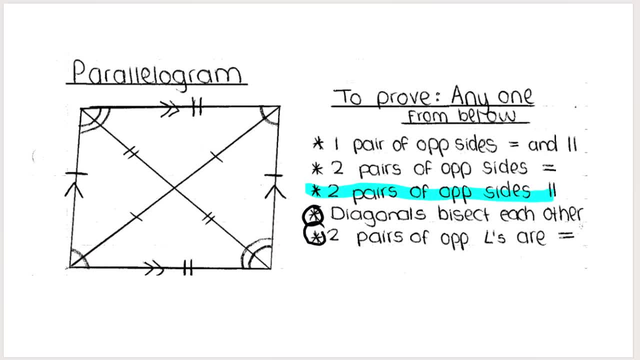 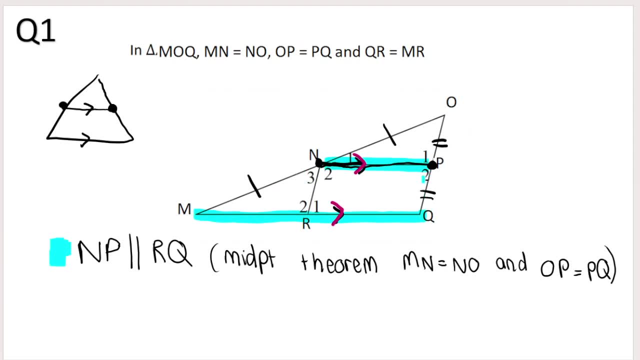 Let's look at the other information they gave us to see if I can use midpoint theorem again, perhaps to prove that the other two sides, nr and pq, are parallel. Remember, they told us not only that mn is equal to no and op is equal to pq, but they 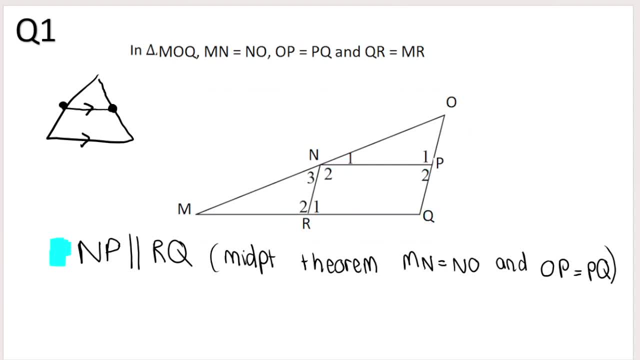 gave us this information as well. So they told us that qr over here is equal to mr, which means that r is the midpoint of that line. And then we also know from previous information, given that mn is equal to no, making n the 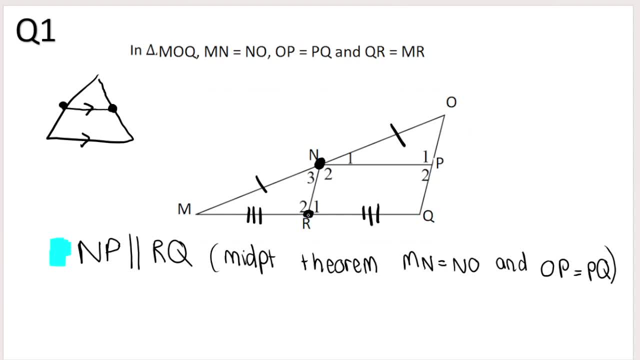 midpoint of that line. I hope you can now see my two midpoints that I've drawn big dots over. If I connect them, that would be the line nr that connects them. What do we know because of the midpoint theorem? Remember, I'm just going to draw a triangle to help. 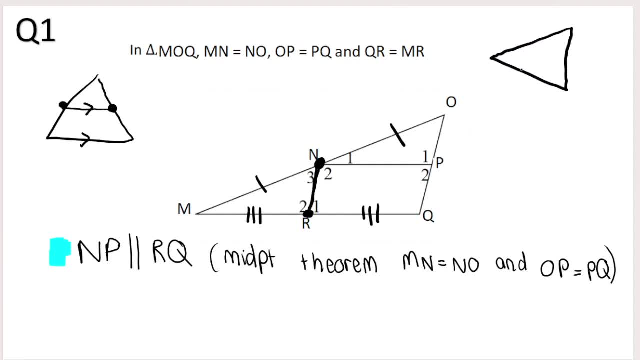 Remember. Mind you, we have now found the midpoints of this line over here. the midpoint of this line, the midpoint of this line. the dots represent the midpoints. If I now join up the midpoints, what can I therefore say about this line over here? and 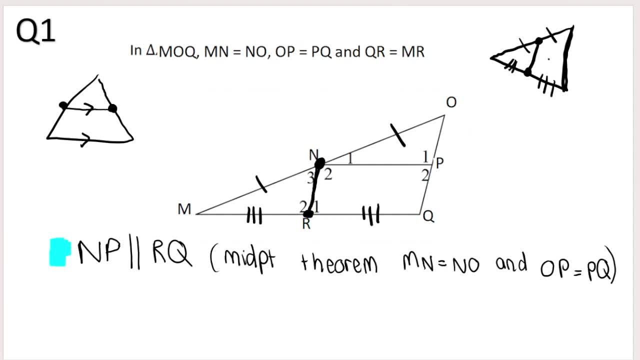 this line at the bottom. Yes, we can say that this line is parallel to this line. So again, I can say that this line over here is parallel to this line and that's perfect, because that's the midpoint of this line. So that then shows us that nr is parallel to pq, and that is the last thing that we 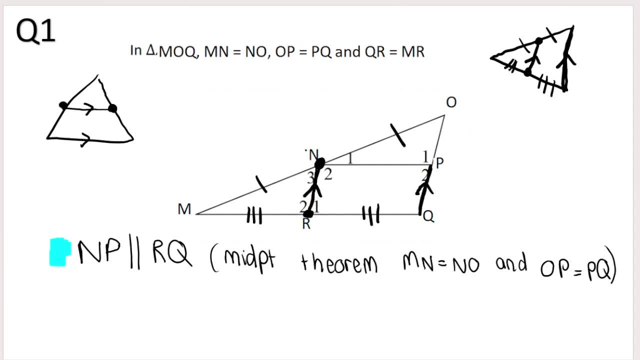 need in order to prove that this shape over here, nrqp is a parallelogram, So I've therefore made another statement: nr is parallel to pq, So the ones are highlighted in yellow And my reason again is midpoint theorem. But take note how I've used different equal lines or different information given in order to conclude. 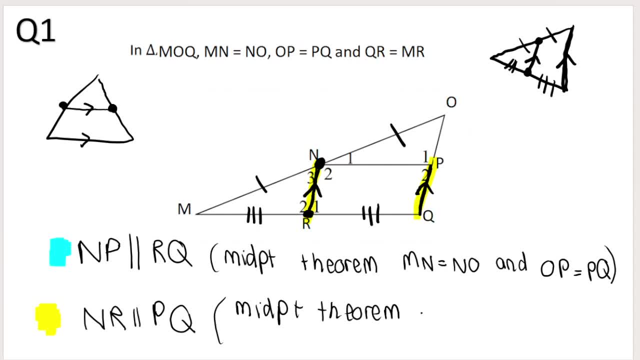 that nr is parallel to pq. So remember, the information that I used in order to conclude that those two lines are parallel was the fact that mn was equal to no same as the first one. giving me that midpoint over there at n, and mr is equal to rq. giving me this midpoint over here. 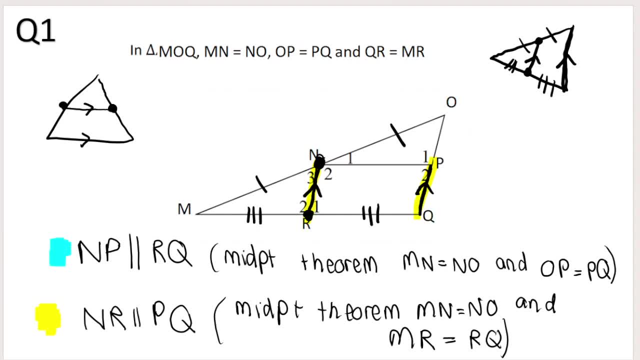 So it is definitely a little confusing. So it is definitely a little confusing. So it is definitely a little confusing Because we've used the midpoint theorem twice, we've used it for on two separate occasions, using two different pieces of information, concluding that two different lines are parallel. 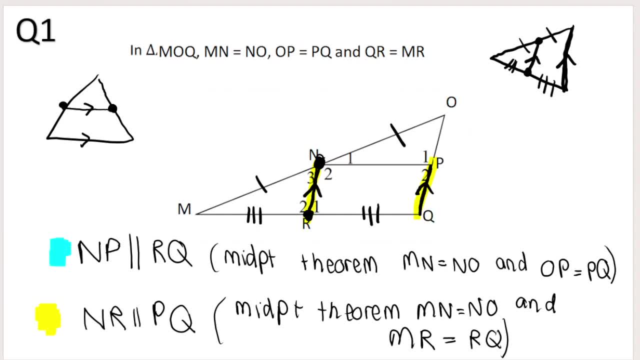 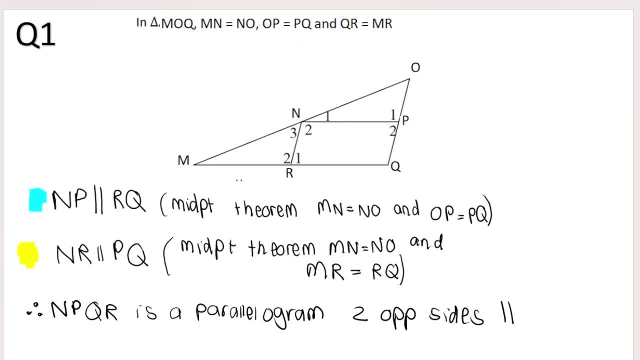 So if you need to go over that again, just make sure you rewind the video, go over it again. But now we've proved that two opposites, two pairs of opposite sides, are parallel. So there's my final statement: npqr is a parallelogram because I have two opposite sides. 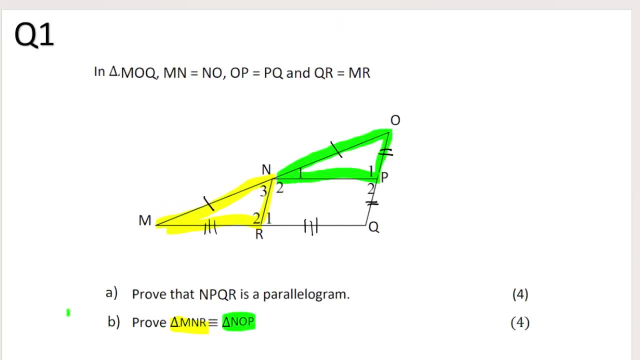 parallel 1b. question 1b wants me to prove that triangle mnr- so I've highlighted that one in yellow- is congruent to triangle nop. Now, first of all, how I remember the difference between congruency, so the congruency symbol. 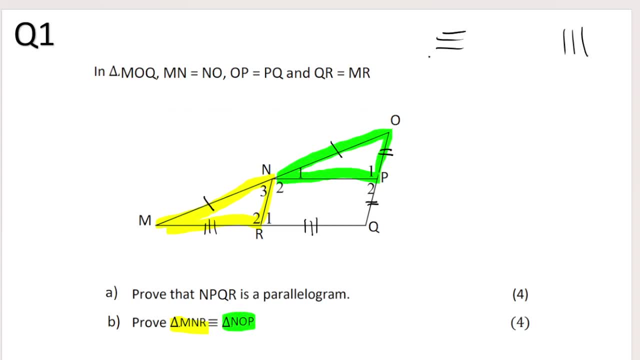 and the similarity symbol is as follows. You should know that congruency means identical, exactly the same, And the way that I remember it is, the congruency symbol kind of looks like a triple equal sign. So, as you know, an equal sign only has two lines. 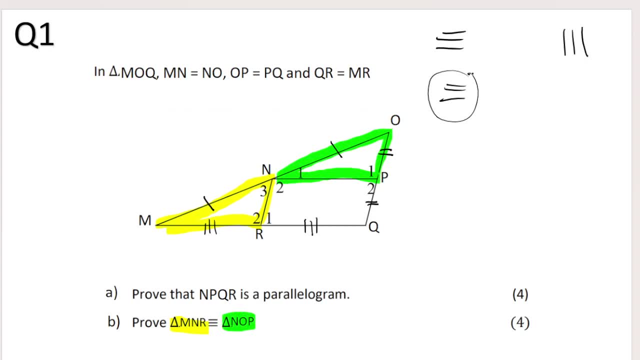 Like that. but congruency has three lines. So triple equal sign, equal, identical, exactly the same. That's how I remember it. So this is asking us to prove congruency, And another thing that should be going through your mind is the different cases for congruency. 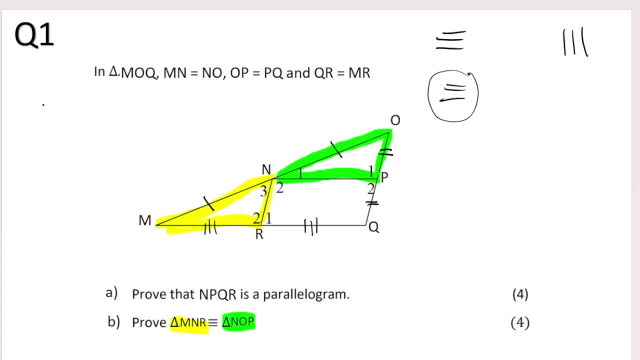 So, in order to prove the two triangles are congruent, we can either use side side side, So showing or proving that all three sides of both triangles are the same, or side angle side, where the angle Proven is in between the two sides that you prove to be equal, or angle angle side, or side angle angle. 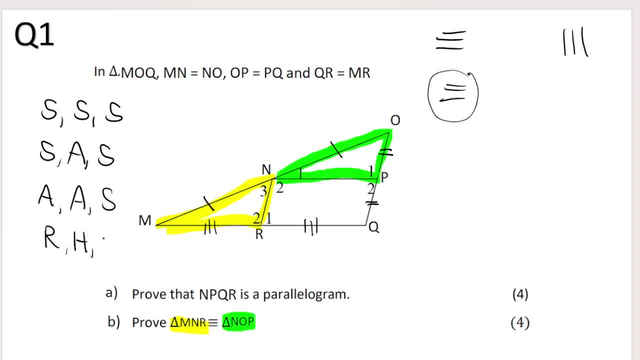 Doesn't matter- or right angle, hypotenuse and side one of these three. So we need to prove that these two triangles, the yellow one and the green one, are congruent, are exactly the same, identical, And I'm going to do that as follows. 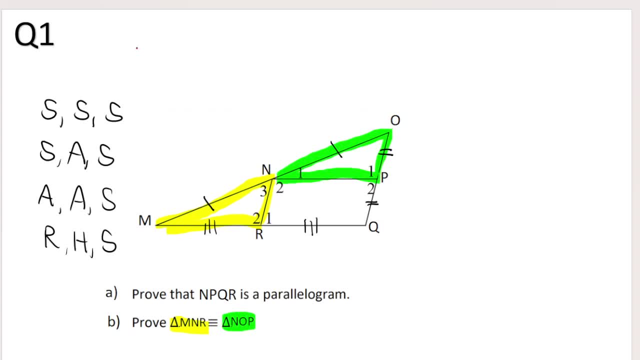 First things first, make sure that all the information that was given in the little right top before and that you Proven in the previous question is on your diagram. so all my equal sides have been filled in. So, for example, MN is equal to NO, and so on. 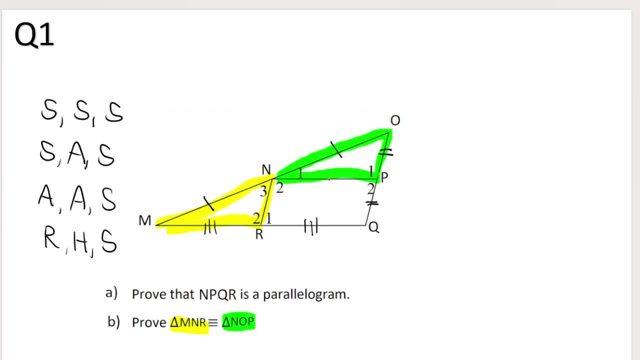 Then in 1A we proved, we showed using the midpoint theorem that NP was parallel to MQ or RQ. So those parallel lines over there. We also showed that OQ or PQ, that line over there is parallel to NR over here. 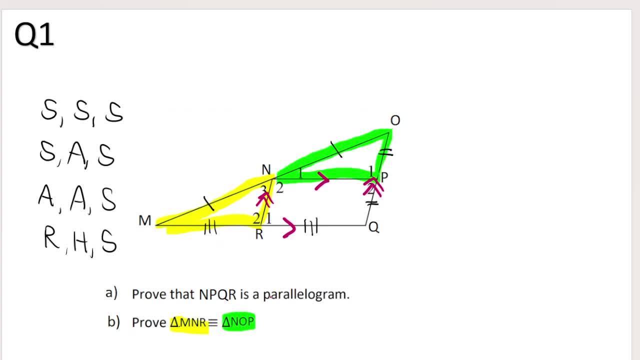 So that may or may not be Useful in the in the question that we're currently doing. So that's very important to fill in. then, another hint or something else that may help you when it comes to proving similarity or congruency is when you're comparing two triangles like that. 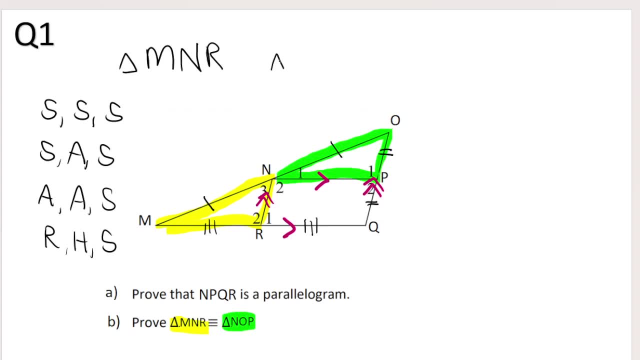 So triangle MNR and triangle NOP. they have been named in a very, very important way. The naming is never, ever random. What that means is because they've been named this way and they're asking us to prove that they're congruent, we're going to. 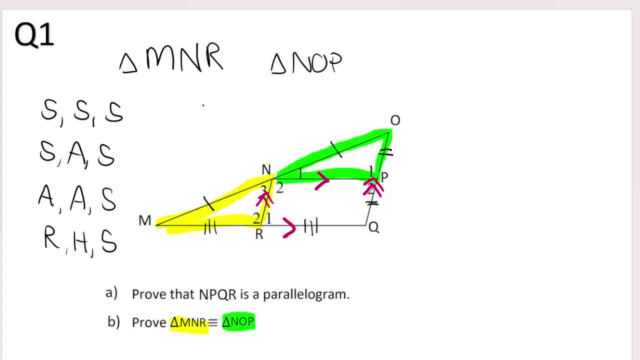 Assume that they are going to end up being congruent. That's why they're asking us to show or prove that they're congruent. You should know that angle M of the yellow triangle should be the same, or will be the same, as angle N of the green triangle. 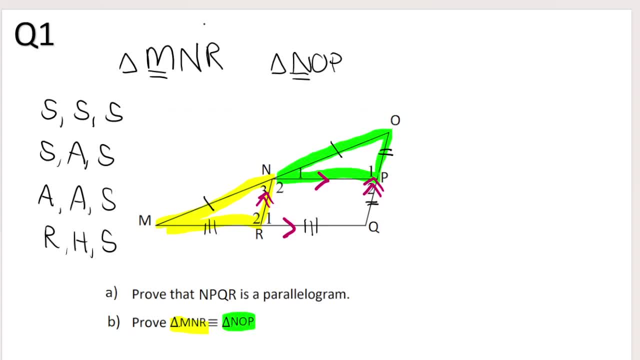 So they should be the same size. So we can therefore look out or look to prove that angle M is equal to angle N or in this case it's angle N1 actually in the green triangle. then angle N should be the same as angle O. 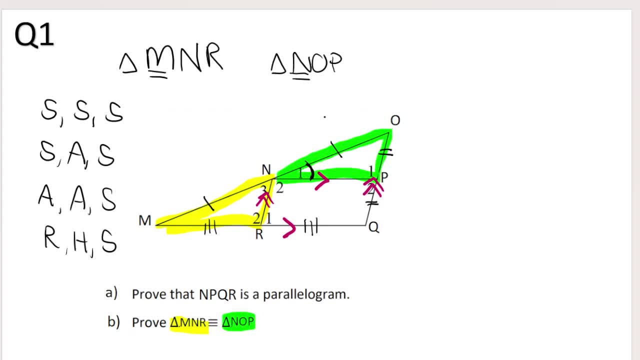 But we're going to have to Prove it or look for clues or reasons on the diagram why we say they're the same and same with R and P, So they're in the same spot in the name of the triangle. for a reason. 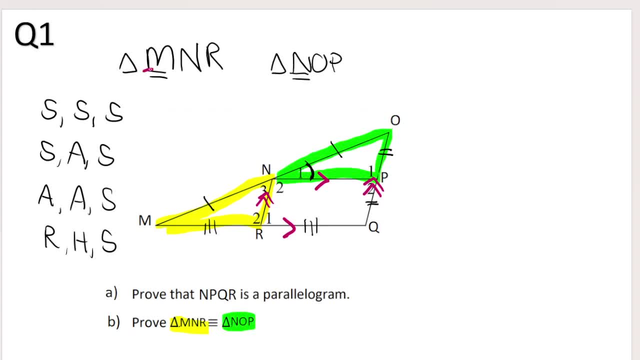 And for that same reason, MN, that's the length of that side. We can try and see if we can prove that it's the same as length. NO, So the first two letters of the first triangle match up with the first two letters of the second triangle. 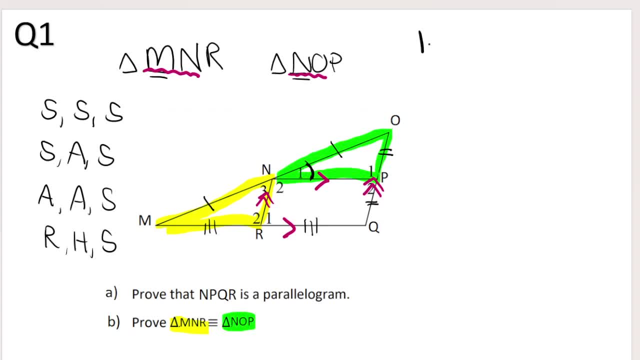 And when I prove congruency. so I'm going to do that now. so I'm going to start off by saying: in Triangle MNR and triangle NOP. So it's kind of like my introduction to my essay, my opening statements. 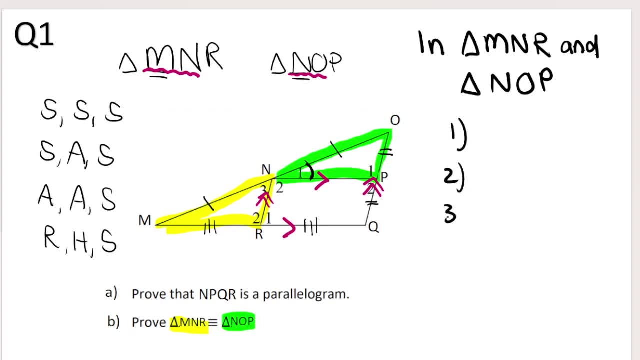 Then I'm going to name, I'm going to look for three reasons to prove that these two triangles are congruent. We need three reasons, You can't just give me two. Look at the cases for congruency: Side side, side side, angle side. 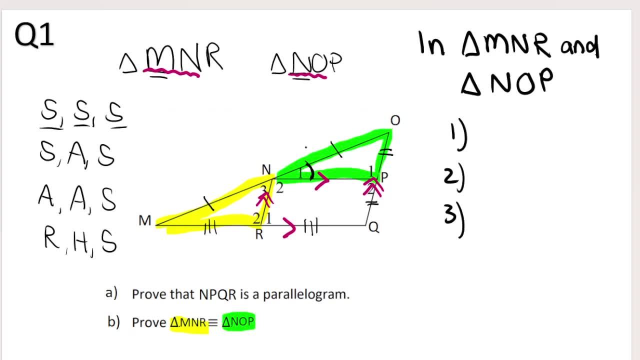 They all have three reasons. You need three reasons. So my first reason, if you look at the yellow triangle, The green triangle, The one that's very obvious to me, is that MN- And they gave this information in the write-up as well- 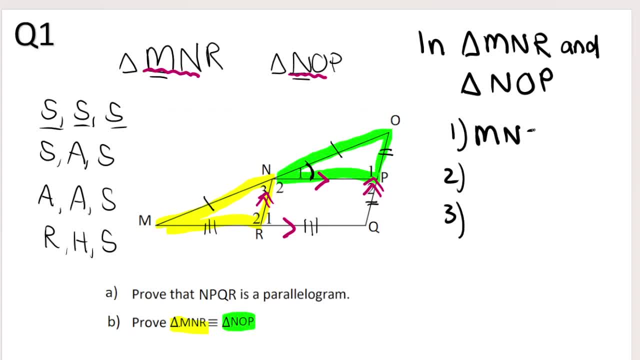 Length MN of the yellow triangle is equal to length NO in the green triangle, And that information was given. So, as you know, in Euclidean it's always statements and reason. My reason is the information was given to me. They gave it in the write-up before. 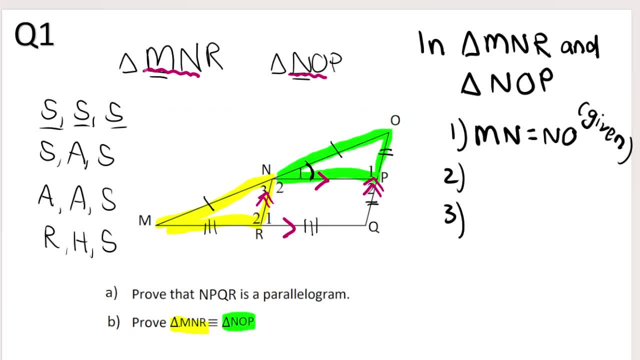 And just to point out what I was saying earlier about the names MN, those two letters are first and second in the yellow triangle's name: MN And then NO. And can you now see that they're the same length? MN is equal to NO. 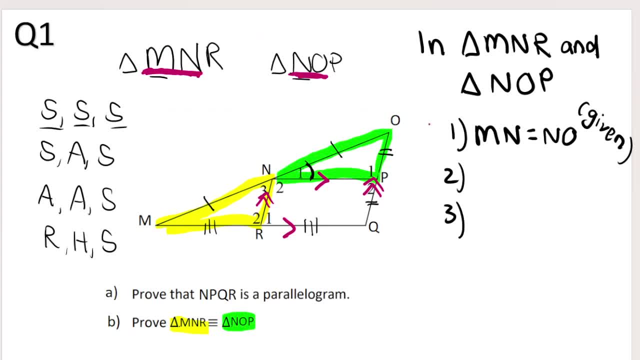 There we go, Done Proven, given That's a side. So I'm just going to make a little mental note here that that is a side. So we've proven that one side is equal to one side. Now if your second reason, if you're looking for another equal side, you're not going to be able to find it. 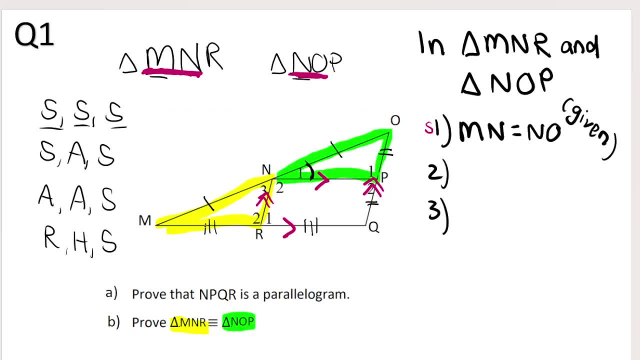 If you look at the yellow triangle, You're going to see that. and also in the information they gave us, they said that MR in the yellow triangle was equal to RQ and RQ is not in the green triangle. You can see- I use three lines to indicate these- that these two sides are equal. 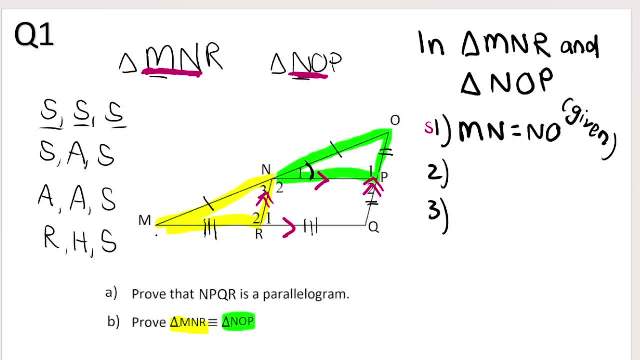 But over here we've got OP. OK, OP is not equal to MR, so we can't use another side. We can't say that NR is equal to anything, because we don't have that information given to us, We can't use it. 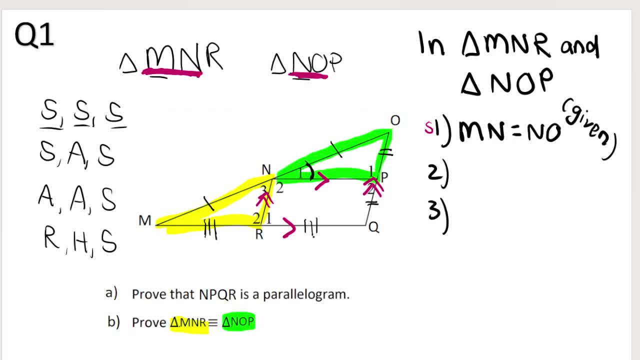 So now we have to start looking out for angles that are the same. Now, if you remember, we drew in that these lines are parallel over here: NP and MR, as well as NR and PQ. So when we have parallel lines, I want you to think of the fun angles. 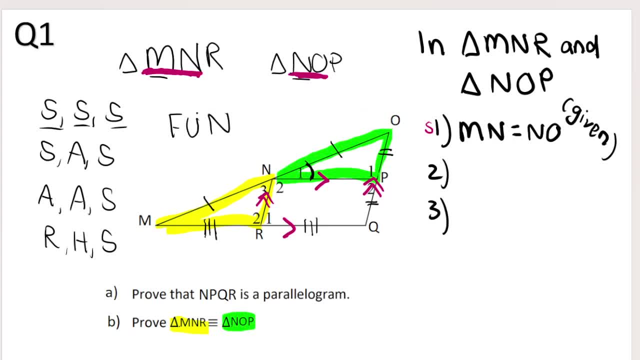 So remember F being for corresponding angles, U being for co-interior angles and N being for alternate angles. Now, if you look very carefully, you can see that we can actually use corresponding angles in this diagram. So let me show you. 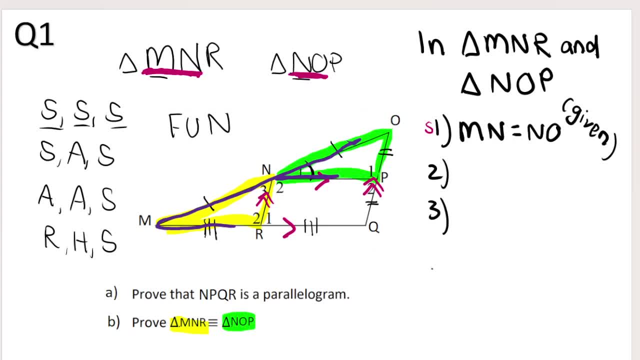 I've highlighted the F in purple. I hope you can see it. It's a very squashed F, but basically it looks like that on the diagram And that tells me that angle M, this angle over here, angle M, is equal to angle N1.. 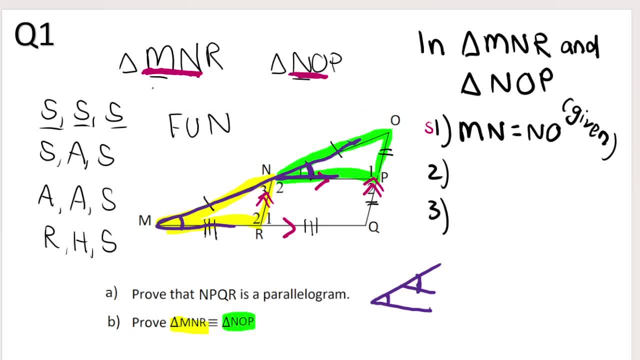 OK, it's over there. So angle M is equal to angle N1.. And my reason for that is corresponding angles. And remember, when you mention any of the fun angles, you have to tell me which lines are parallel. So corresponding angles. 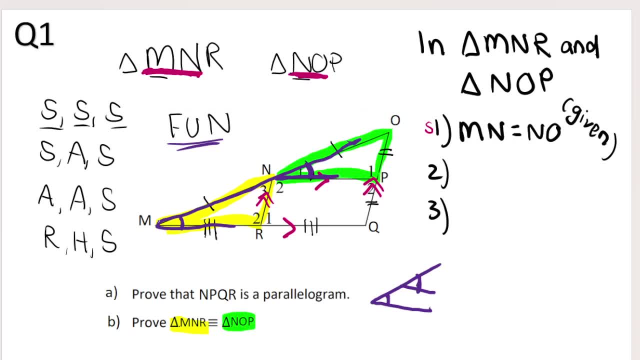 And then you will say: NP is parallel to RQ or MQ. There we go. Angle M is equal to angle N1. You cannot just say angle N, because, as you can see, we have angle N1,, we have angle N2,. 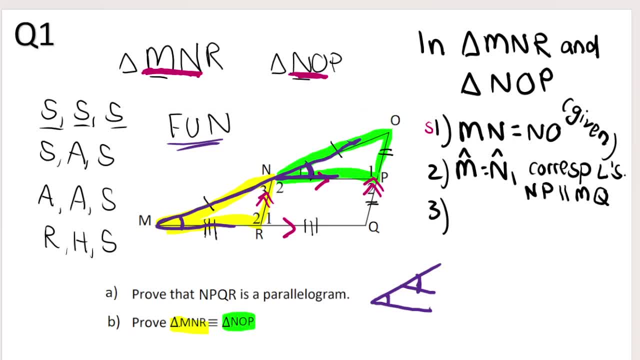 we have angle N3, so you have to be specific And then we say corresponding angles and always mention your parallel lines. Now we need one more reason. So reason one was a side side. So MN being a side is equal to NO being a side. then angle M is equal to angle N1.. 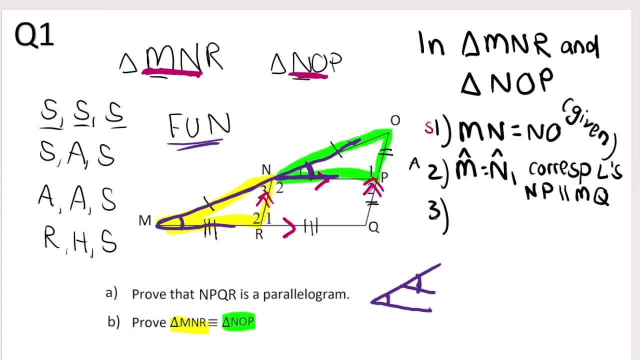 So this was a angle. Now we're going to look for another angle, because we already concluded that we can't find any more equal sides. So remember not only these two lines that were just highlighted in purple, not only were those parallel, but we also had this line. 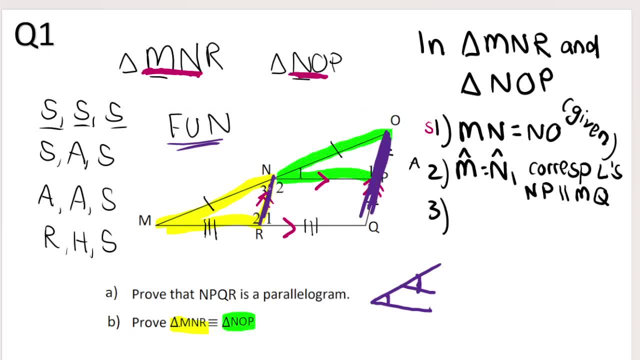 Sorry, I'm drawing it in so thick just so that you can see it being parallel to this line and therefore I can find an F going that way as well. That tells me that angle N3 over here is equal to angle O. So what I've done now is I've drawn an F as well, but it's kind of leaning on its. 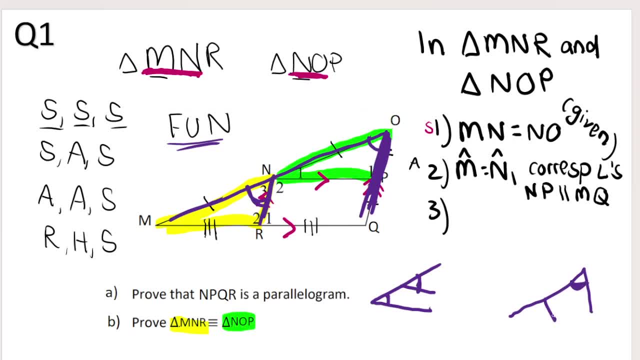 side like that. So angle O in the green triangle is equal to angle N3 in the yellow triangle, And again that's corresponding angles. But just take note that your parallel lines will not be the same set of parallel lines you used in reason number two. 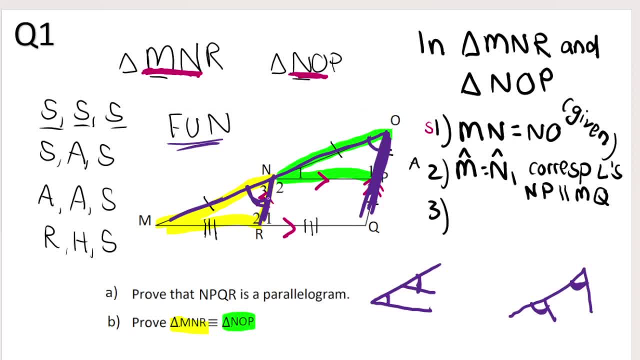 It'll now be that NR- this line over here, NR is equal to OQ this line over here. So different set of parallel lines. So now I've got my three reasons in order to prove that the triangles are congruent. so therefore, you conclude by saying: triangle MNR. 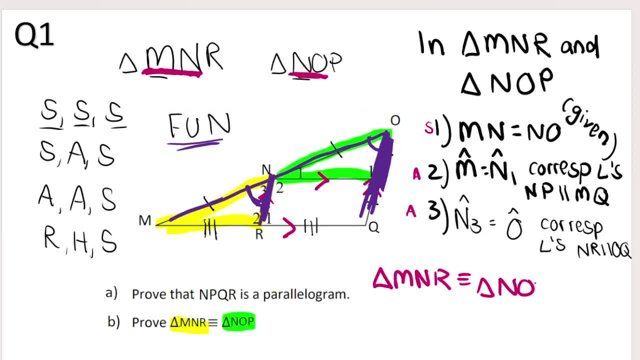 is congruent to triangle NOP and your reason is side angle angle. You can also say side angle angle means exactly the same thing. Why is it side angle angle? Well, because reason one was side, reason two and reason three were angles. We showed that angles were equal. therefore they are congruent. 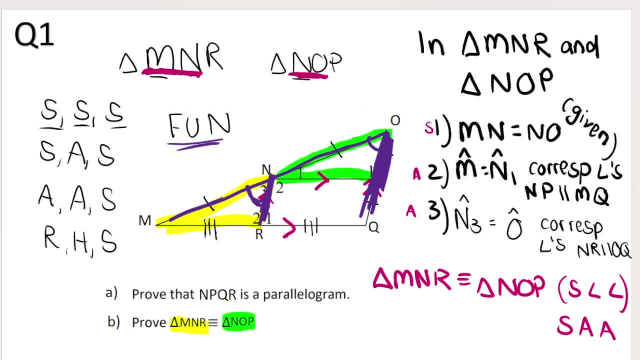 And now, because they are congruent, we can therefore conclude the following: The other angles that are equal. So we can say, for example, that angle R2, this one over here, angle R2, is equal to angle P, which is actually over here, P1,. 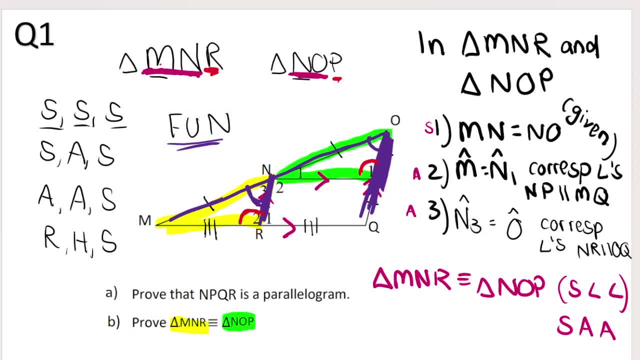 just a little bit under my purple mess over here. We can also say that we remember. we said that MN was equal to NO. We can therefore also conclude that NR is equal to OP, stuff like that. So once you've proved that they're congruent, then you can match up the other. 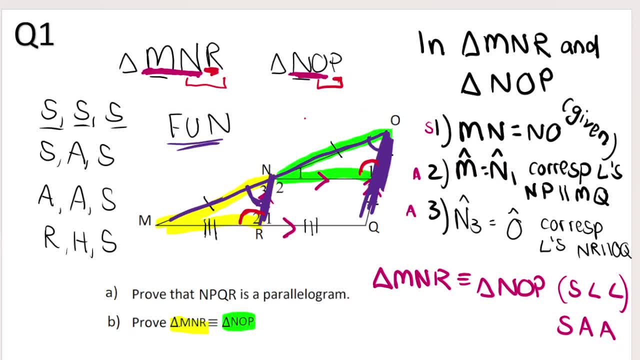 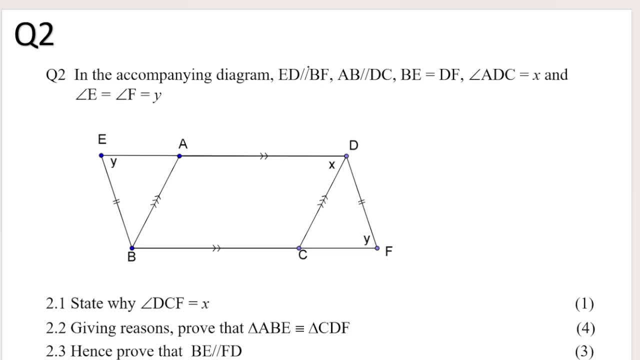 letters to say what other sides are equal and what other angles are equal. Question number two says in the accompanying diagram ED is parallel to BF. that's already indicated on the diagram We've got. no, it's actually not. EB is parallel to BF. 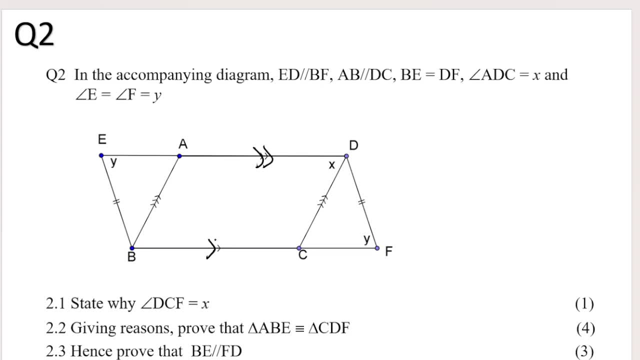 Yes, it is. it's just very light ED parallel to BF. so we got that. AB is parallel to DC. Again, we've got that over there. AB and DC, We've got. BE is equal to DF. we've got that. 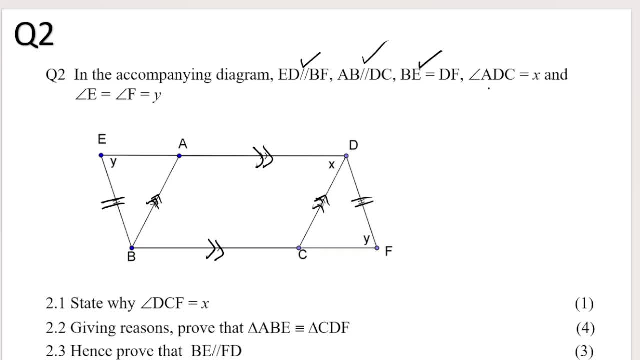 already. We've got angle ADC, so we would write it like: that is equal to X, that's over there. And angle E is equal to angle F, which is Y. OK, cool, So they're giving me that that is equal to that which is Y. 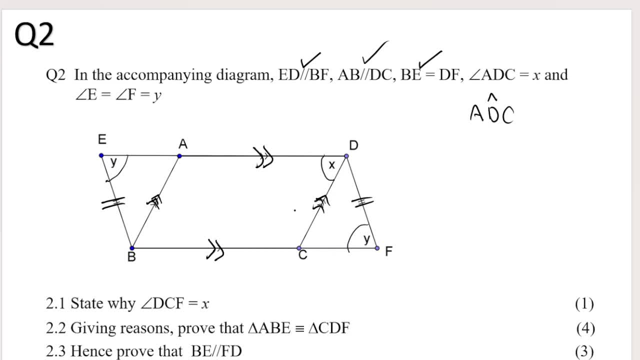 State Y, angle DCF is equal to X. So they are asking us to state Y, this angle, angle DCF, That's this angle over here. How do we know? We know that that is also equal to X. Well, I can see it immediately. 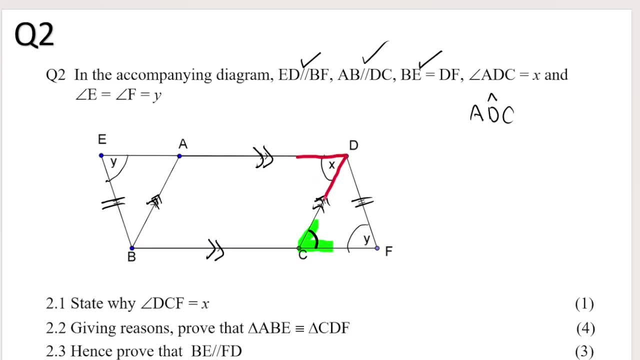 I hope you can see it- the Z or the N over there. And we know that that is alternate angles, alt angles, And when we mention one of the fun angles we have to mention parallel lines. So 2.1 will be that X or angle. 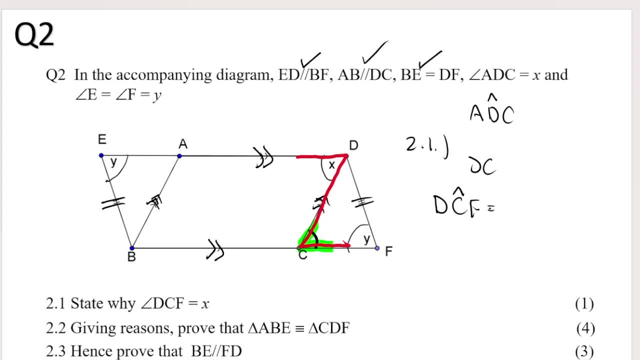 DCF is equal to X. The reason is alt angles, and the parallel lines That we used would be: this one is parallel to this one which they gave us at the beginning. they told us that ED was parallel to BF. There we go, There's your answer for 2.1.. 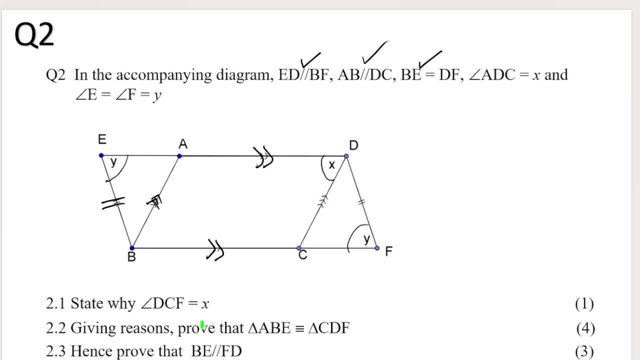 Question 2.2 says giving reasons, and we must always give reasons- Prove that triangle ABE- that's this one over here, I'm going to highlight it in green for you- is congruent to triangle CDF. Going to highlight that one in yellow for you. 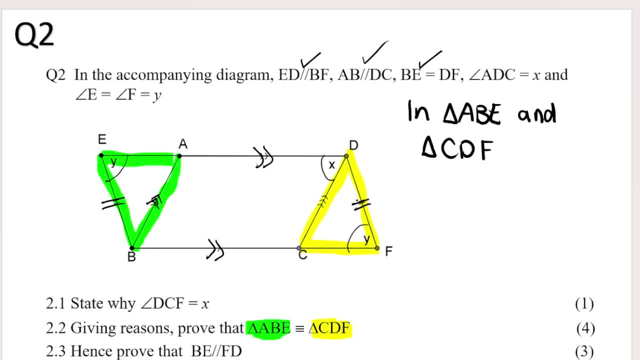 OK, so proving congruency again, let's start off. So, starting off, I'm just going to make sure that all the information that I have written before the diagram and that I've already proven is indicated on the diagram. So remember, we found in question 2.1 that angle DCF was equal to X. 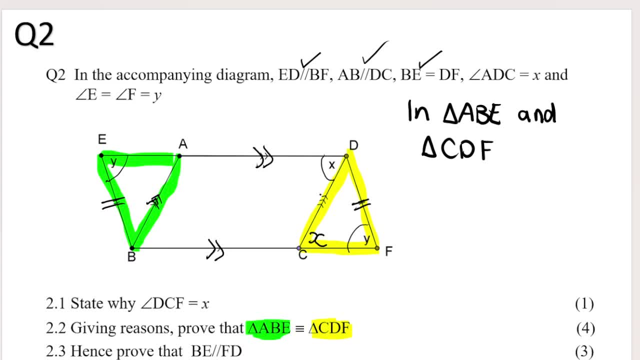 So I'm just going to fill that in over there. That may or may not help us later on, And that's all I have for now. So I start off by saying: in triangle ABE and triangle CDF. it's just a nice way to start off your. 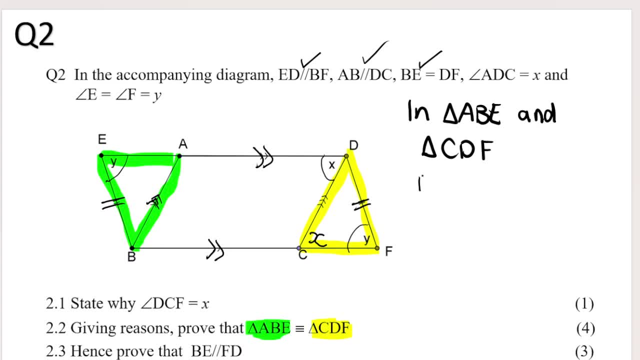 congruency and similarity when you prove it. And then we're going to have three reasons: Number one, number two, number three. Number one: I can immediately see that angle angle. Let's start over here. angle E: Angle E in my green triangle is equal to angle F in my yellow triangle. 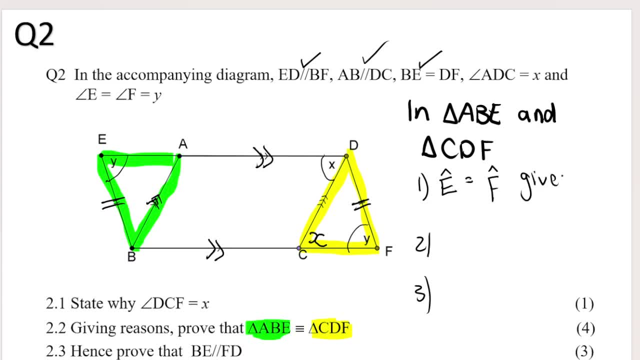 And my reason for that is, given that information was given to me in the right up over here And it was also indicated on the diagram below. They're both equal to Y. So there we go. That's given information, And just please take note how I'm naming it in this case. 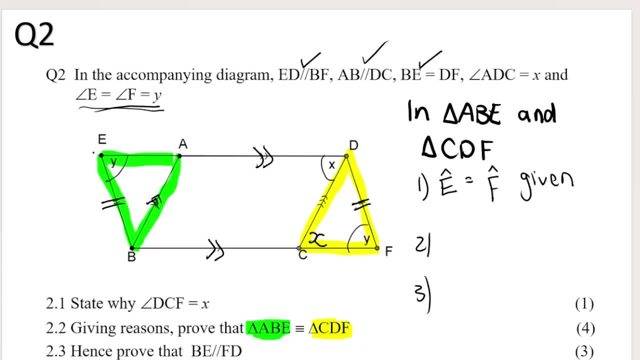 I'm saying angle E and angle F in this case And I'm not saying, for example, angle AEB or angle BEA or whatever, because they can only really be one angle when referring to angle E. It's just this one over here. 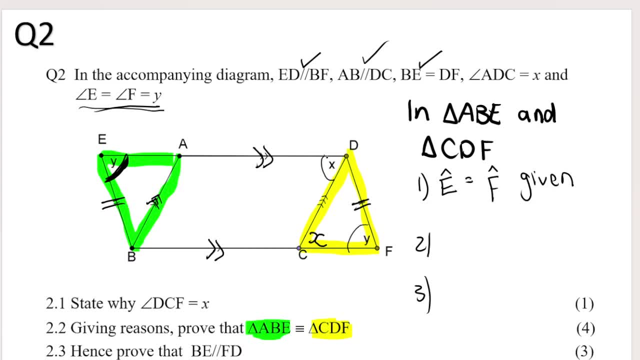 Same thing for angle F. But if I were to name this angle over here, this one over here where the X originally was, I would have to say ADC or CDA. The reason why is because there's another angle over here involving D. 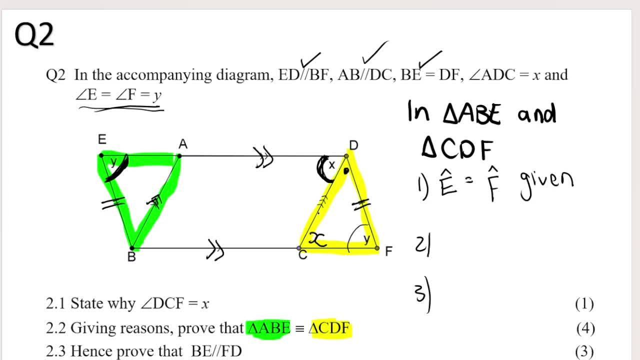 involving that corner, that vertex, So that's why I have to name that in a very specific way. I hope that makes sense. OK, back to proving. So that is an angle that I've mentioned over there. Then the other thing that I immediately 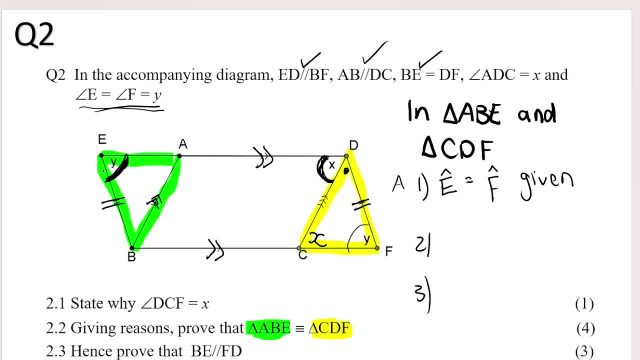 see that is also given is the fact of these two sides here being equal. So I can say that BE side, BE that side over there, is equal to side DF. OK, it was given. given in the right top. given on the diagram. 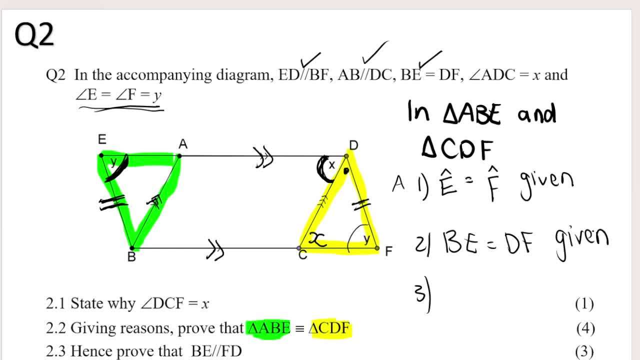 So I'm going to say, given, Now I need one more piece of information. So that was a side. So it's either going to be an angle or it's going to be a side. We do not have any information to go with another side. 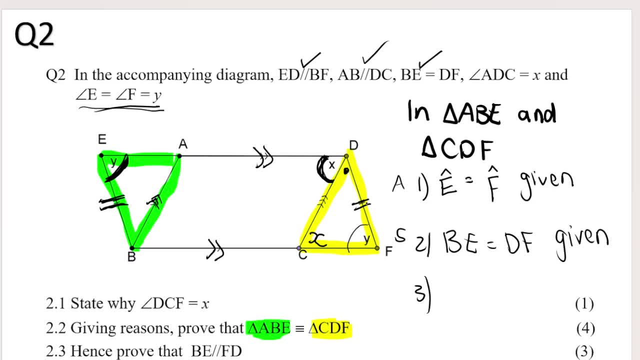 We were just given the information of BE being equal to DF. I don't know anything about the other side, So let's look out for another angle. This triangle over here, the green one, doesn't have any information at the moment about an X angle. 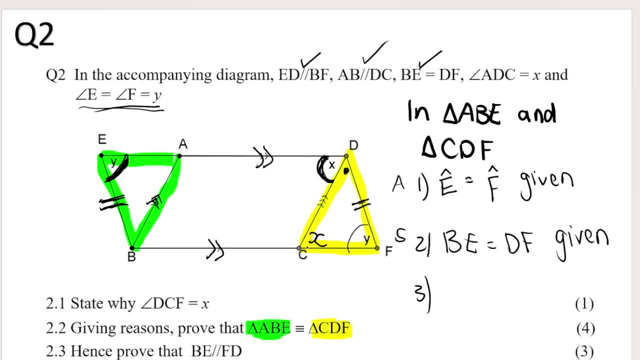 Can you see? the yellow triangle over here has angle DCF being equal to X, But I don't have anything in the green triangle about an angle being equal to X. However, we can use information, other information on the diagram, to show that there's another angle that is also equal to X. 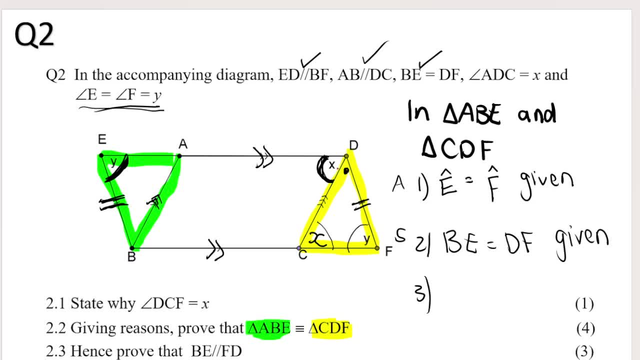 So I hope that you can see what I'm seeing. But this line over here, this one over here, is parallel to this line over here- Information that was both written above and indicated on the diagram. So if I join those two I can create an F. 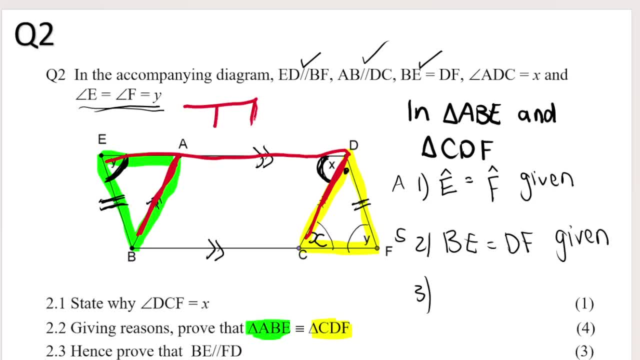 So basically, what you're seeing at the moment is an F lying sideways, like that. We know that this angle over here is X, So if that angle is X over there because of corresponding angles, this angle over here must also be X, which means this angle over here. 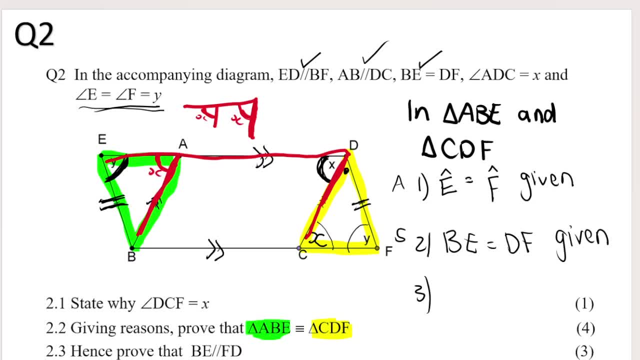 must also be X. And what are we going to call that angle? Remember, we can't just say angle A. We can't just say angle A because there's also this that's also there by A, So let's call this BAE. 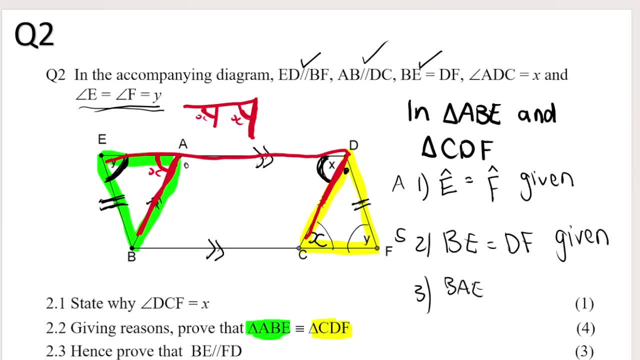 So I'm first going to say over here that B angle BAE is equal to X as well. Why? Because of corresponding angles, Corresponding angles, And remember to mention your parallel lines. So that would be: AB is parallel to DC. So now that we mentioned that, angle BAE is equal to X. 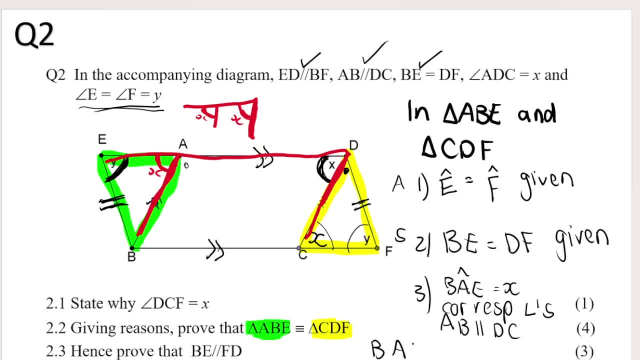 we can therefore say that angle BAE is equal to angle DCF, because they're both equal to X. Sorry, DCF, There we go. OK, so there we go. And that's all because of corresponding angles. That's why angle BAE is equal to X and therefore they're both equal to each. 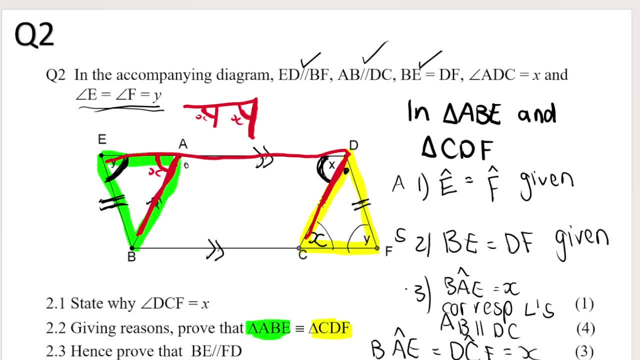 other, because they're both equal to X. That's my third reason over there, And that again is an angle. So we've got side angle angle or angle angle side. So therefore, my final statement- Now I've run out of space over here. 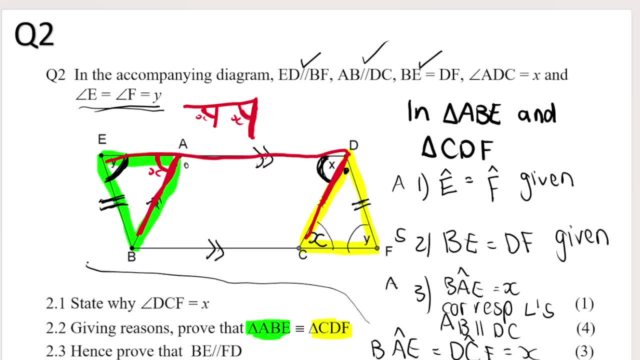 but imagine that what I'm doing over here is continuing at the bottom. So I'm going to say: therefore, triangle AB is congruent to triangle CDF And I used side angle angle. There we go, Or angle angle side, doesn't matter. 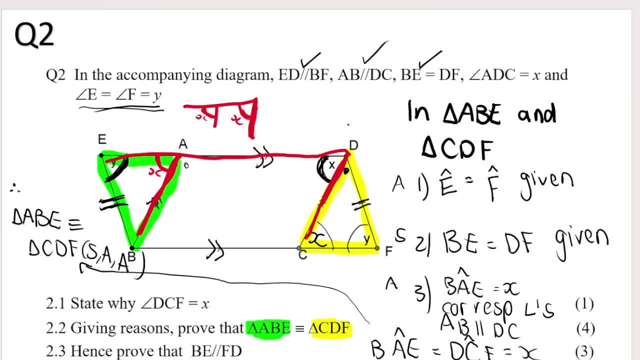 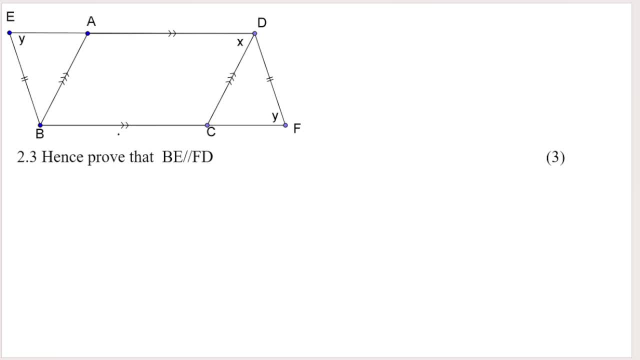 Just remember that this final statement over there must come underneath my three reasons. My next question, 2.3, says: hence prove that BAE is parallel to FD. So they want me to prove that this line over here, BAE is parallel to FD. 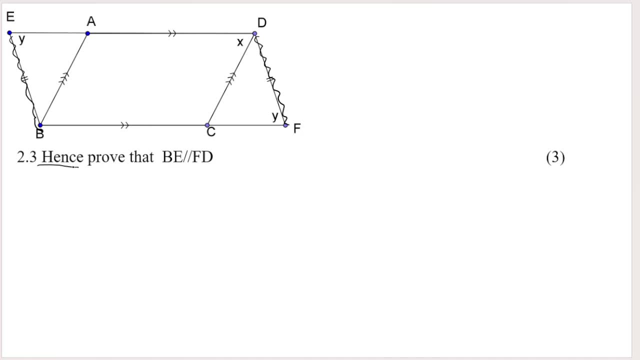 Right Now. when they say hence, it's kind of like they're asking you to follow on from your conclusion or from what you've proved in your previous question. therefore, because of what you just proved, or following on from what you just proved Now, can you please prove the following: 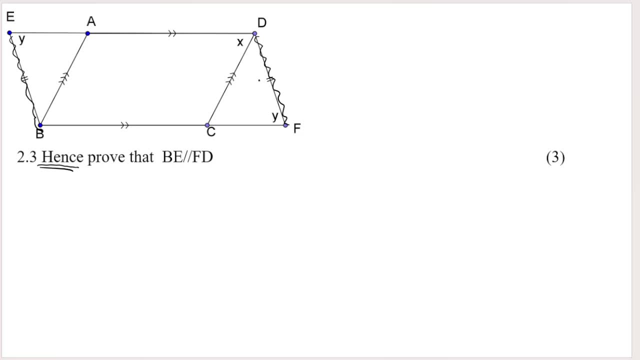 So I'm going to do two ways in which you can do this. Remember, in Euclidean geometry it's very, very nice in that there's often multiple ways to get to the correct answer, As long as you give your statements correctly, with correct reasons, that is. 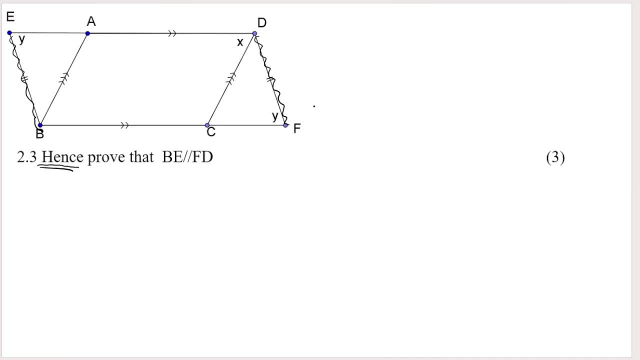 paired with that correct statement, you will be awarded all your marks. So I'm going to show you two different ways and you can decide which one you like better. Let me know in the comments below which one you preferred for method 2.3. 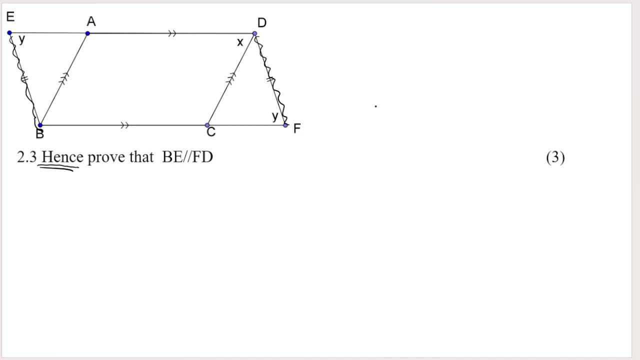 for question 2.3.. So you can just say method one or method two. But let's go, I'm going to do method one right now. So method one. So the first thing that I'm going to say is I'm going to say: 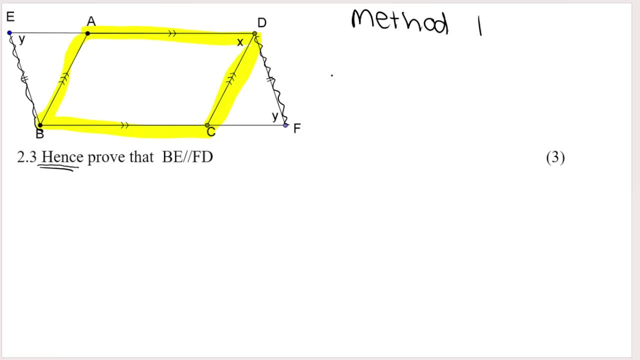 So we know- And this is from information already given to us- that AD is parallel to BC. That's, given information That is the top line over there- is parallel to BC. We also know that AB is parallel to DC. 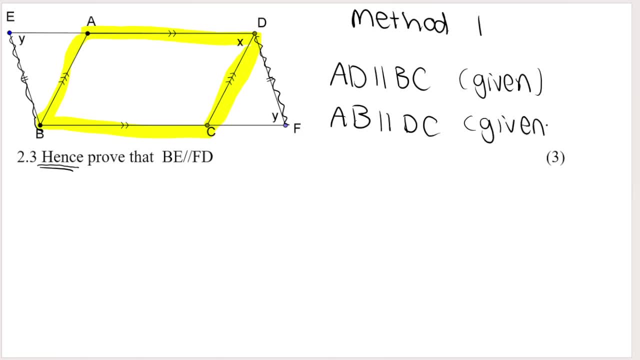 Again, that's given information. So that is this line over here. AB is parallel to DC. Now what do we know about the fact that if we have two opposite sides that we have shown or proven to be parallel, we can therefore conclude that in ABCD? 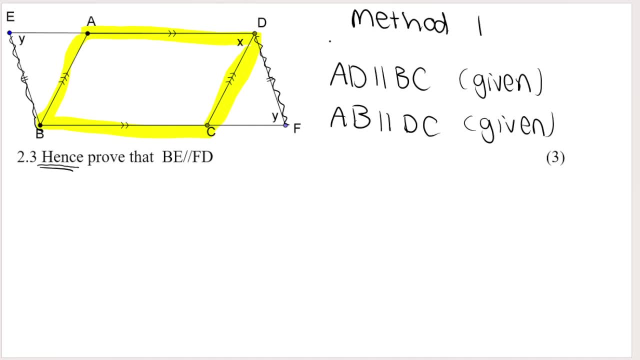 ABCD is in fact a parallelogram. So I should have started off by saying: in ABCD, the following pairs of lines are parallel. Therefore, ABCD is a parallelogram. Two opposite sides parallel. 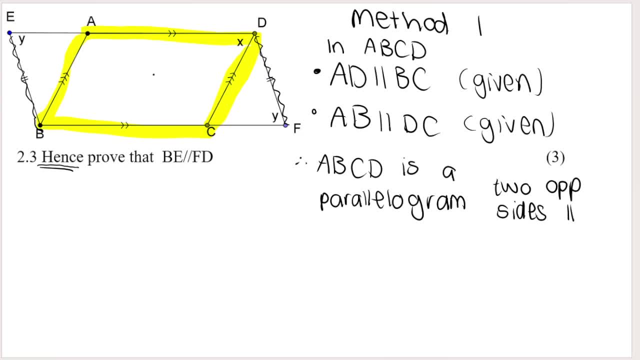 That's my reason. Two opposite sides or two pairs of opposite sides are parallel. Then the other thing that I know: I know that AE is equal to CF, And the reason I know that is because what I proved in the previous question, that's why they say hence: 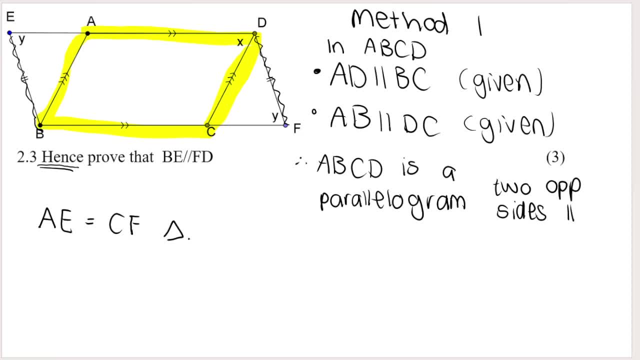 using that previous information, and that previous information was that triangle ABE is congruent to triangle CDF. And remember what I said just a little while ago. I said that ABCD is a parallelogram. So if you look at the length of this triangle, 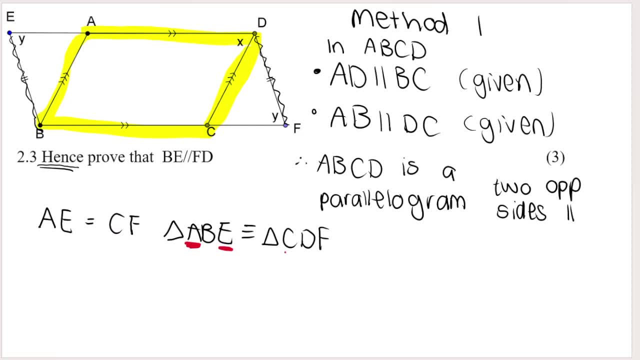 ABCD is equal to triangle CDF. So if you look at the length of this triangle, that side ABCD, that side AE- because they are congruent, because they are identical- will match up with CF. 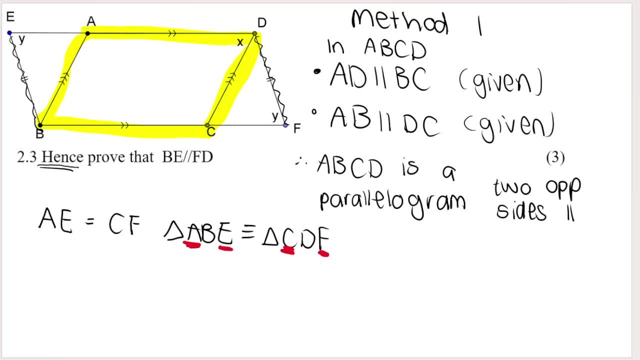 In other words, the length of AE will be exactly the same, will be equal to the length of CF, because they are congruent triangles. OK, so we know that those are equal. So, basically, what we're saying is that this side 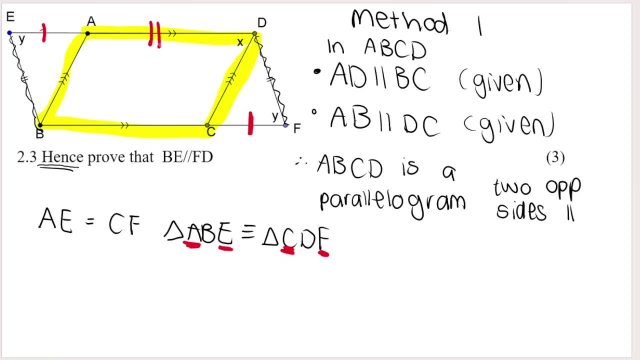 b c. d is a parallelogram. is that a? d will be equal to b c? i hope you see where i'm going with this. a d is equal to b c. do you see how i've given my reason? opposite sides of palm parallelogram. 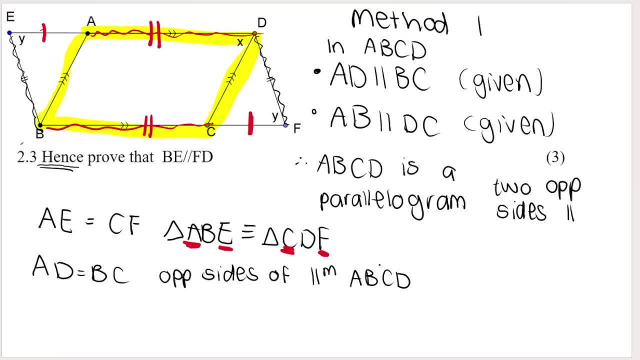 a, b, c, d are equal. so that's my reason. the opposite sides of parallelogram, a, b, c, d, e, a, b, c, d are equal. so basically what i know now is that because a- e is equal to c, f- okay, stated over there- and a- d. 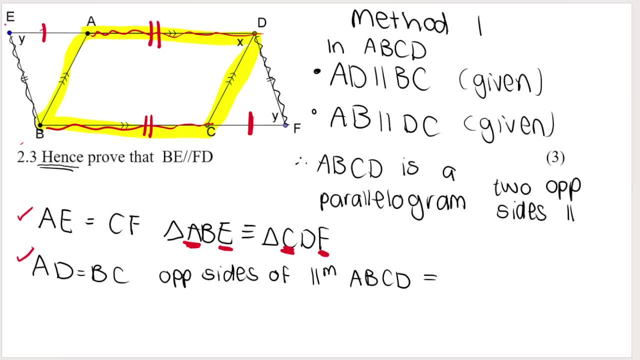 is equal to b c, as stated over there. what that tells me is that this entire side over here is equal to this entire side over here that i've mentioned over there. therefore, e, d, so that entire side over there is equal to b f, that entire side over there. now, remember, i hope you can see that. 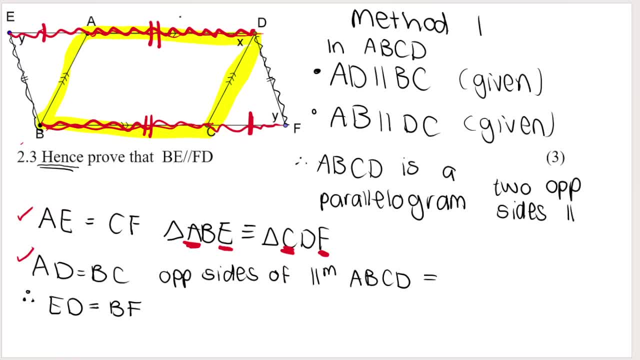 what i'm trying to do is i'm trying to show that this big shape over here- b e d f, the big one- is a parallelogram. remember, up here i have shown or i've proven that the yellow one is a parallelogram. but if i can show that the big one b e d f, that big one, if i can show that that is also a. 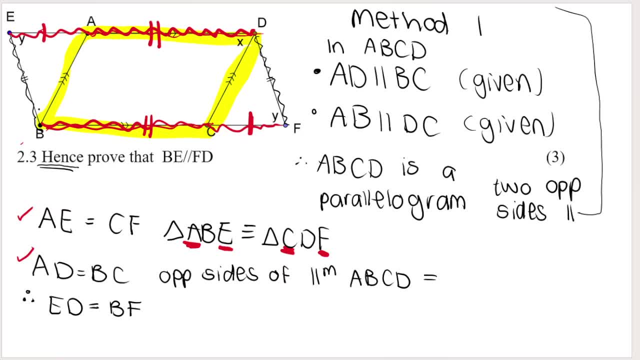 parallelogram, then i can conclude that b? e is parallel to d? f, which is what the question wants. so i'm almost there with proving that the big one, the big shape, b e, d f- is a parallelogram. so i've shown now that one pair of opposite sides 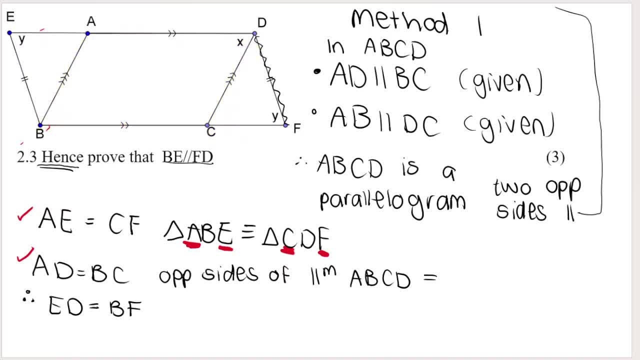 are equal. so i've shown- let me use a highlighter- i've shown that this side is equal to this side because of the two congruent triangles. i've shown that this side is equal to this side because of the fact that a, b, c, d is a parallelogram. so what i've shown so far is that this side is equal in. 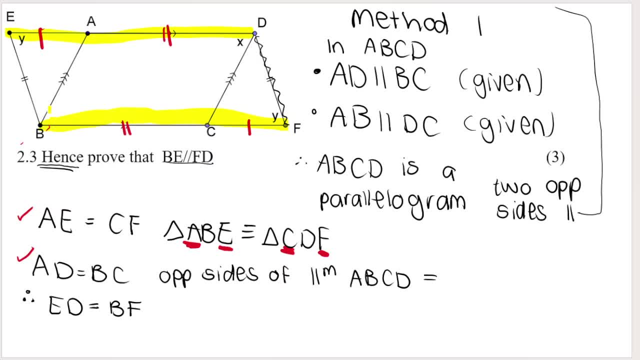 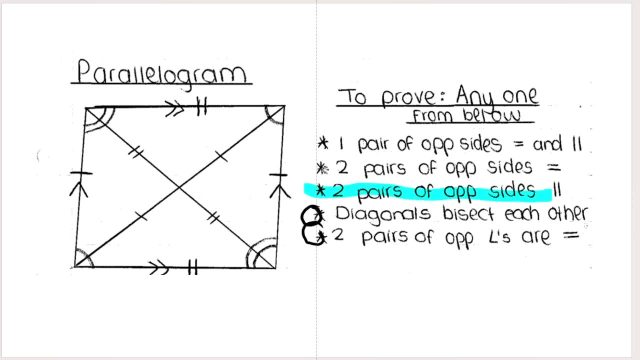 length to this side. so i've got one pair of opposite sides being equal. but remember, in order to prove that a quadrilateral is a parallelogram by using equal sides, i need to show that two pairs of opposite sides are equal. see over here. i need to show two pairs, so i've shown one. let's see if we can see the other side. 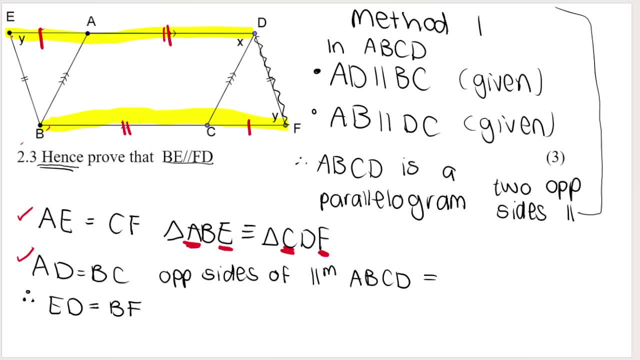 so basically, what i'm saying is: i now need to prove that this side is equal to this side, and look at what they've given me in the beginning of the question and on the diagram. in the writing, they've already told me that e b is equal to d f, so therefore, 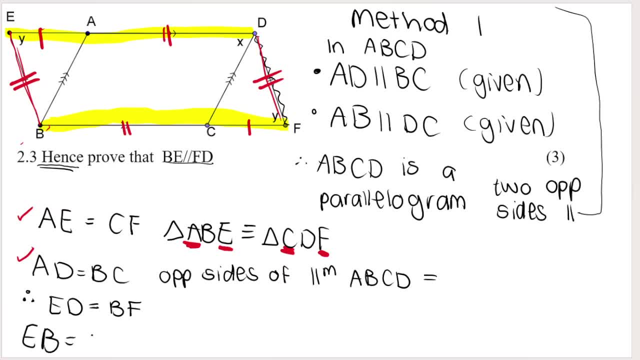 we know e b is equal to d f. that information was given. so now we basically know that two pairs of opposite sides are equal in the big parallelogram. so i'm going to carry on on the next slide, therefore, because i now have two opposite sides being parallel and being equal, i 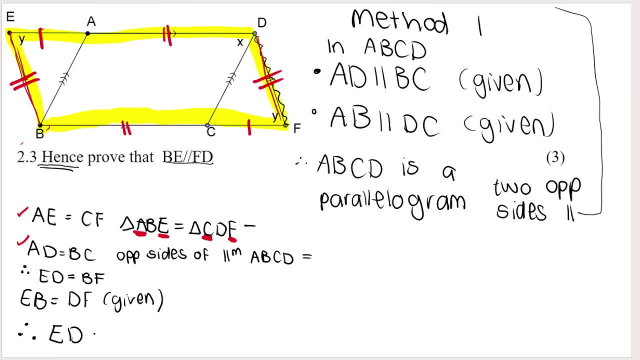 can say that e, d, e, d, f, b is a parallelogram, and my reason for that is because i've just shown, or i've just proven, that two opposite sides are equal, and because i've now shown that it's a parallelogram, my final conclusion is that e b or b e 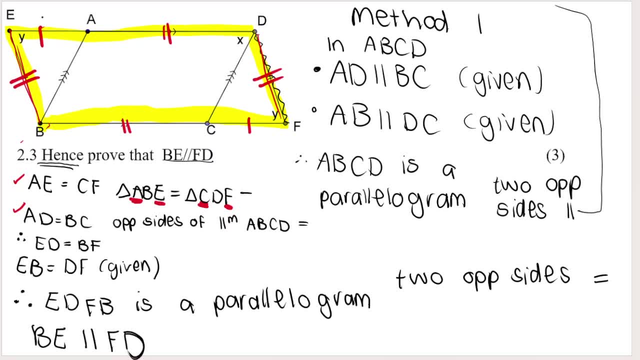 is parallel to f d. so because i've shown that this big yellow thing is in fact a parallelogram, i can therefore say that this pair of opposite sides is parallel. okay, it is a bit long. there's a lot that you have to show. remember, for every statement you must give a reason. so let's go to. 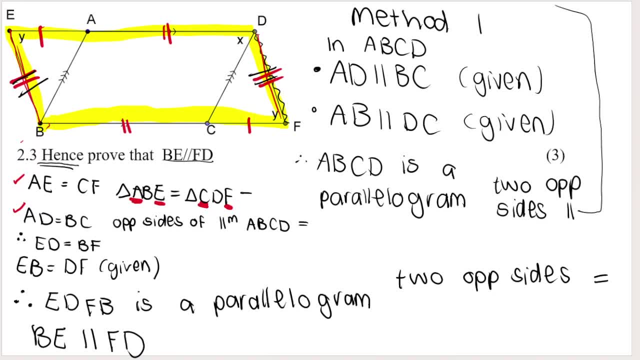 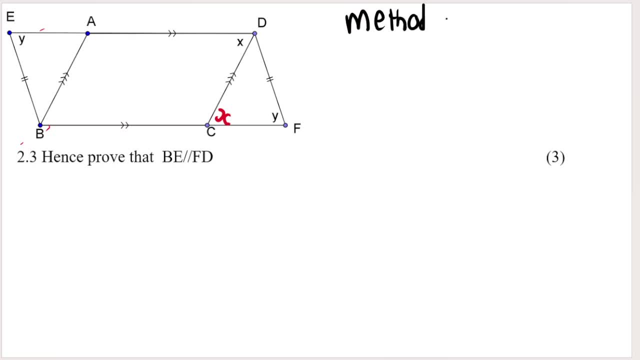 method two, which i think a lot of you would actually prefer. now, in method two, i'm going to work more with the angles and i'm almost going to use a converse of one of our theorems that you've You've already been taught. one of our reasons is that you've already been taught to show that these lines are parallel. 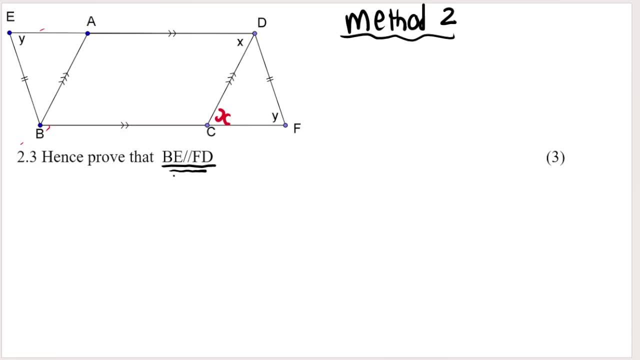 So, just as a way to start this off, remember we can only use fun angles, So corresponding angles, co-interior angles, alternate angles, if we know that two lines are parallel. But if I can do the following, if I can say, okay, here's some random lines. 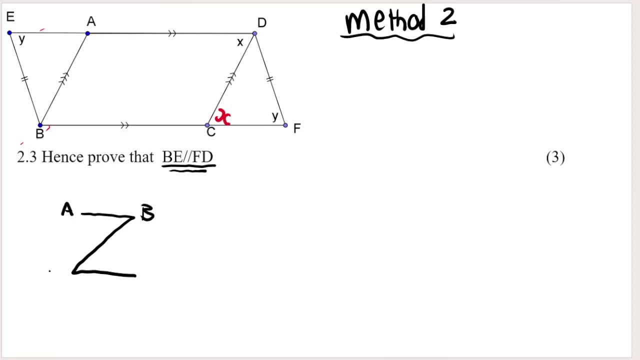 Let's say that I can say that this is A, B, C and D And I give you this angle over here as being X. or let's say, actually this is 20, and this is 20 over here, If you can tell me that angle ABC is equal to 20, and that's equal to angle BCD, which is equal to 20.. 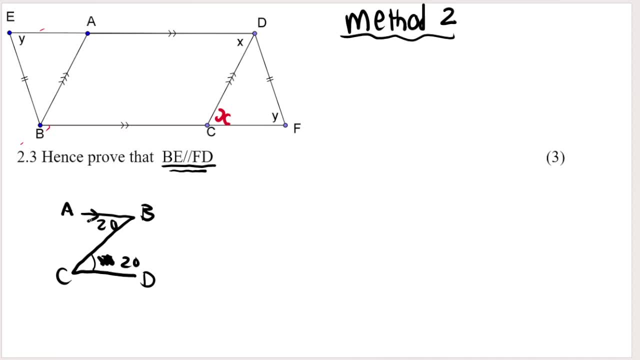 Therefore, from that information- because these angles are equal- we can conclude that AB is parallel to CD, So it's basically the converse. So by showing that the angles are equal, we are saying, therefore, it must be true that those lines are parallel. 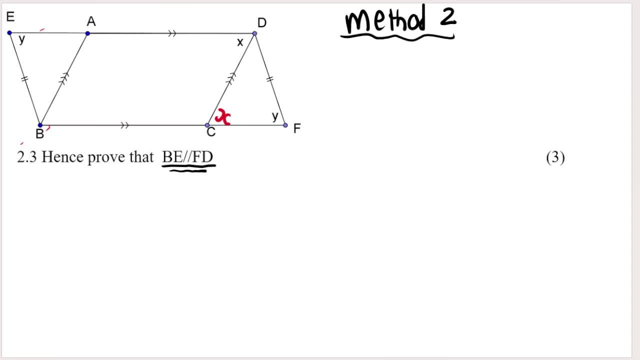 So we're going to basically use something very similar in this question, And this is actually what the memo of this particular paper did do. So method one was a reason that I went with. This is what the paper's memo did, But I find this to be a very cool method: much shorter, actually using angles. 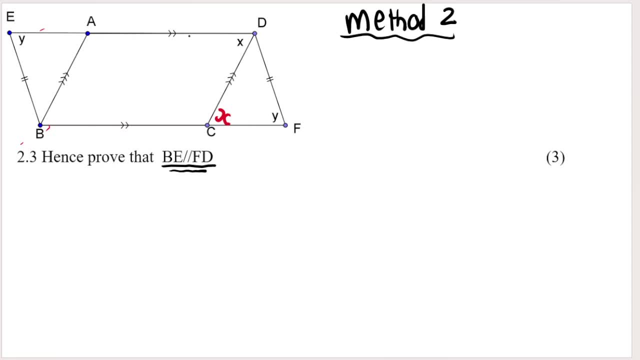 So first thing that I'm going to do is I need to prove that this line over here B E, this one over here, is parallel to FD over here. Now, if I want to prove that those lines are parallel, I could think about co-interior angles. 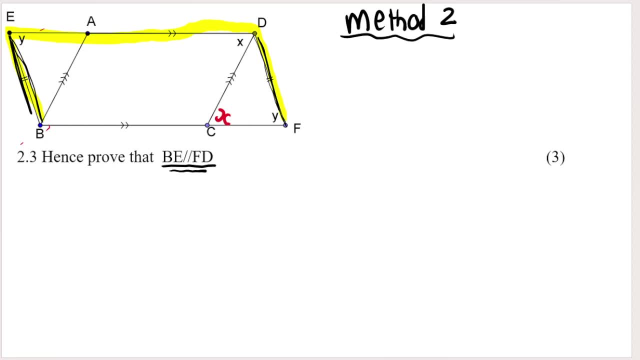 This is how the thought process works, if you want to use this method. So, in order for co-interior angles to work, if the lines are parallel, then what will happen is this angle over here, which is angle E, or angle BED, Will equal to this angle. 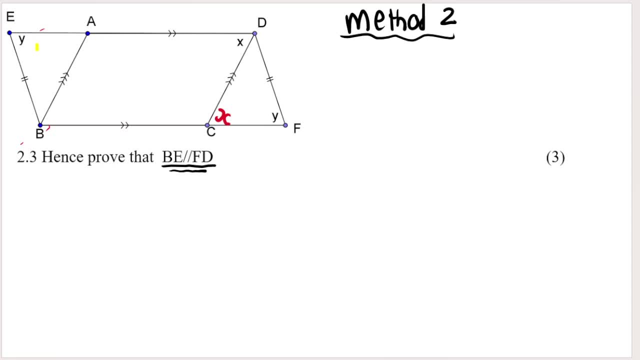 So this is kind of a thought pattern or the thought process that you can use in order to implement this method. We want to prove that this line over here is parallel to this line, So I hope that you are already thinking along the lines of co-interior angles. 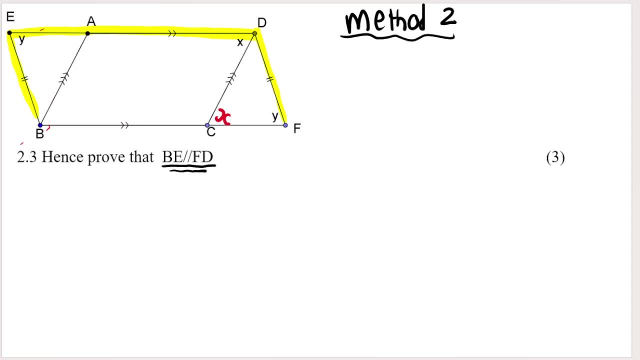 And I hope you remember that, in order for co-interior angles to be true, in order for that to work out. So remember, co-interior angles is the U or the U, and it basically says that these two angles, the sum of these two angles, will give me 180. 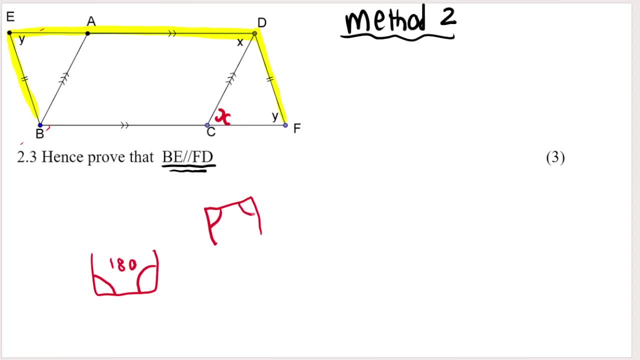 So co-interior angles are supplementary. If you add up those two angles together you're going to get 180.. So basically, if I can show that this angle over here, which is angle B, E, A or BED or angle E, whatever, this one over here, 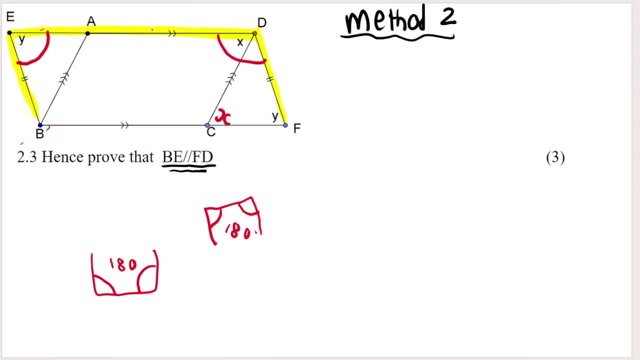 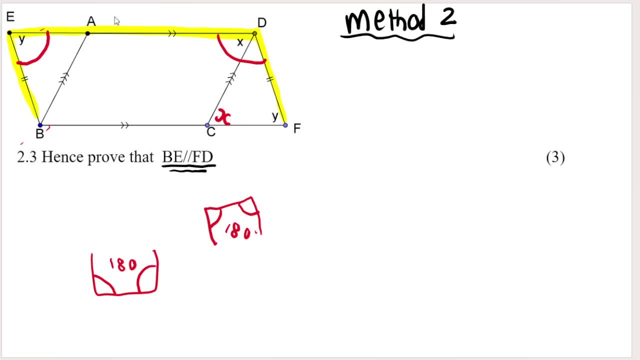 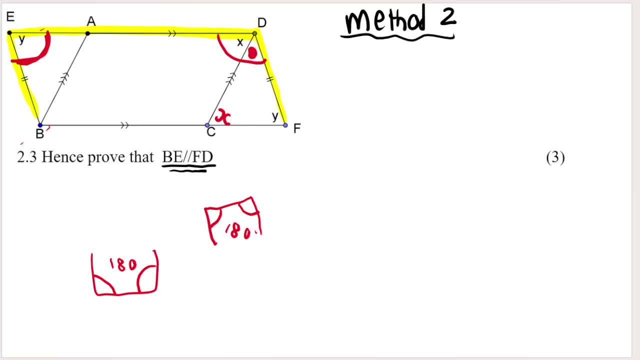 So my first step is: I'm going to try and find this angle over there. So I'm going to try and find the following angle: angle CDF. That's what I'm going to try and find first. So what I know is X. 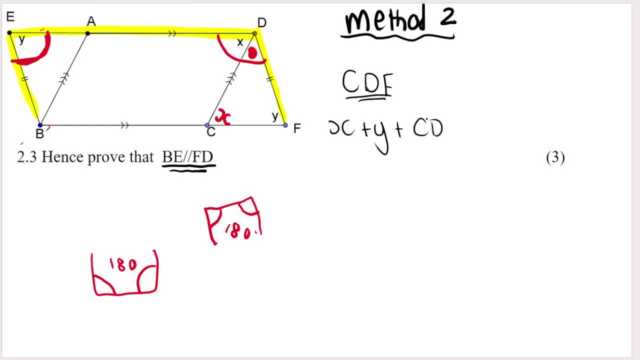 Plus Y plus angle CDF, must give me 180.. Okay, so angle X- this one over here, plus angle Y plus angle CDF, which is this one over here, must give me 180.. And my reason for that is: angle sum triangle CDF. 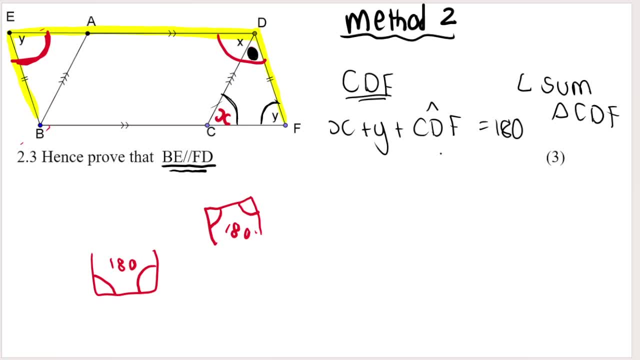 So the sum of angles, the sum of the angles in triangle, CDF, that means the following Angle: CDF Is equal to 180 minus X minus Y. So that angle is 180 minus X minus Y, this one over here. 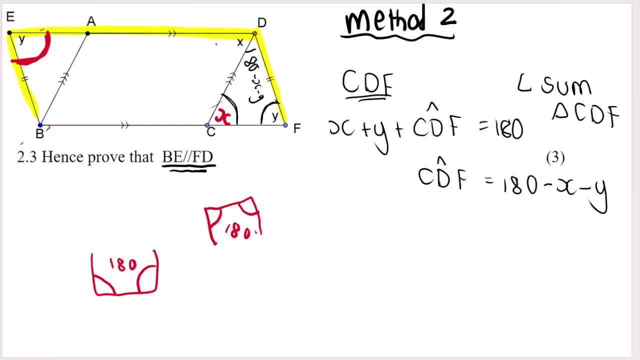 Then what I can say is: angle EDF, In other words this big one over here, this entire angle over here is therefore, so I'm just going to write: angle EDF Is therefore X. Okay, So this part over here. 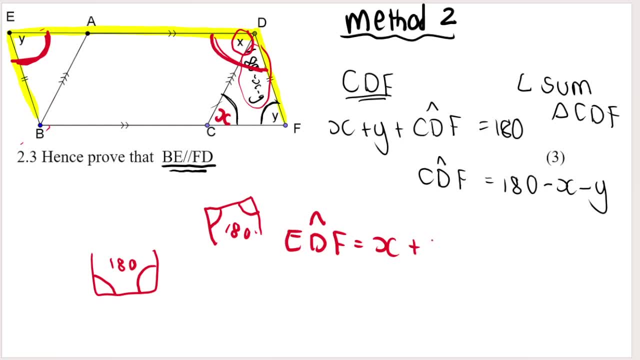 Plus 180 minus X minus Y. If you simplify that, you'll get angle EDF As being 180 minus Y. So I hope you can see what I've been doing over here. So I have found just to make this clearer. I have found the size of this little angle over here. 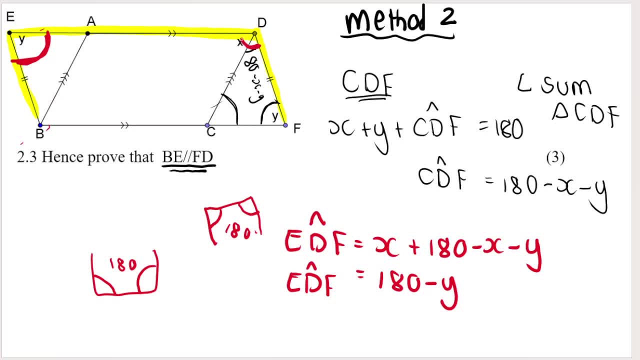 That is 180 minus X minus Y. Okay, So this is 180 minus X minus Y. Then I'm adding this angle over here, which is X. So the sum of those two angles together, if that's X and this one is 180 minus X minus Y, then the sum of those together is 180 minus Y. 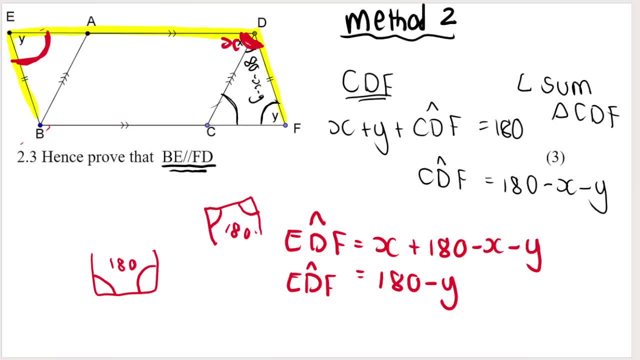 Then what I'm going to do is I'm going to say, okay, cool, If I take angle EDF and I add this angle over here which we're going to call angle E, What is that going to get me? Angle EDF. 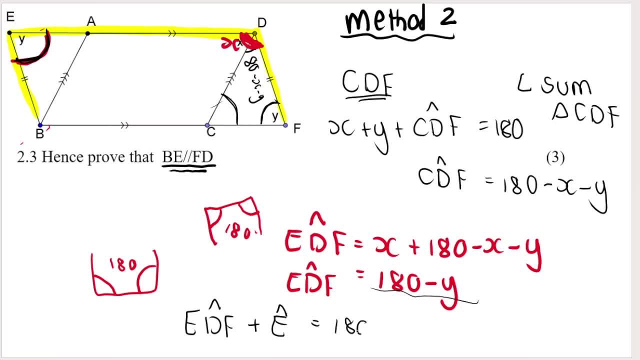 Angle EDF is this one over here: 180 minus Y, And I'm going to add angle E, which is Y, And I hope you can see what I'm going to get: 180 minus Y plus Y, Minus Y plus Y. 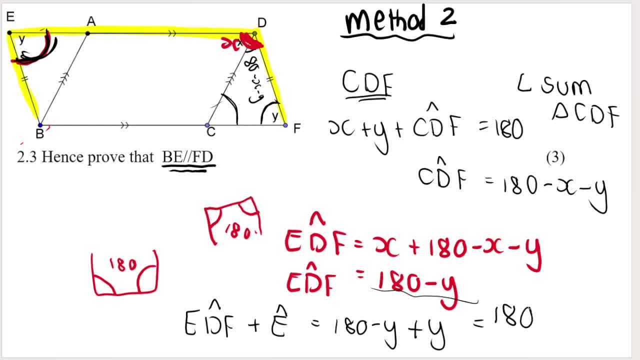 Those cancel, Those go away. So I'm going to get 180.. So basically what I'm saying is inside my U shape over here: these two supplementary angles, this one plus this one, When I add them together I get 180. 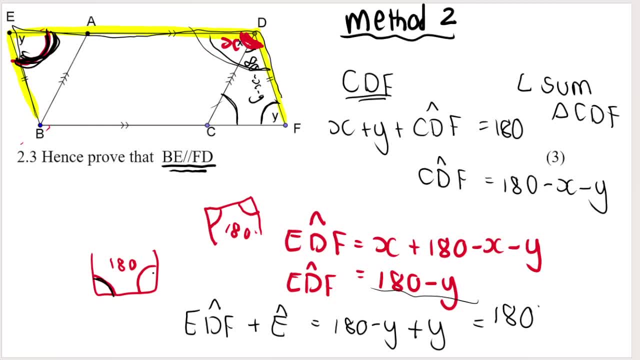 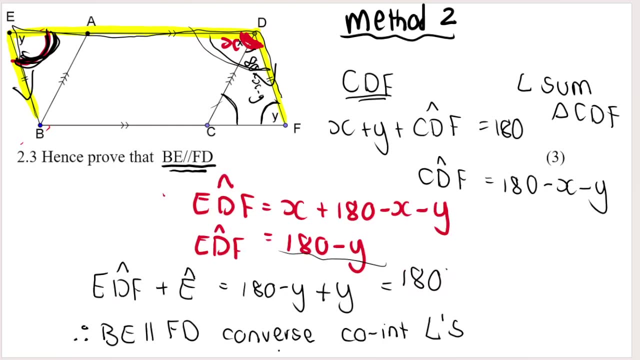 And what did we say If the Co-interior angles, or the inside angles over here, add up to 180,? we said that we can therefore conclude that these two lines are parallel. We can therefore conclude that BE is parallel to FD. And what I did is I use converse co-interior angles. 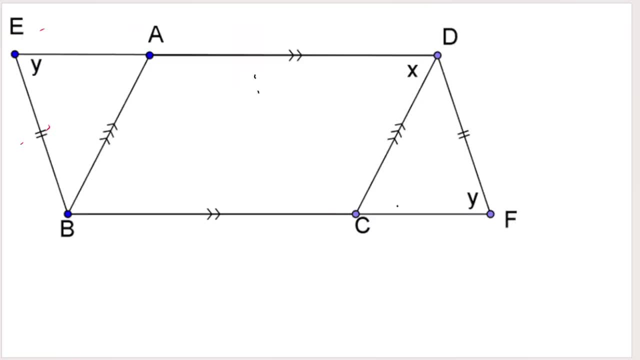 So, just to recap, here's a bigger version of what I just did Remember: DCF was equal to X, as we showed in the first question. This angle, Because X plus Y plus this angle would equal 180.. So I'm going to add 180.. 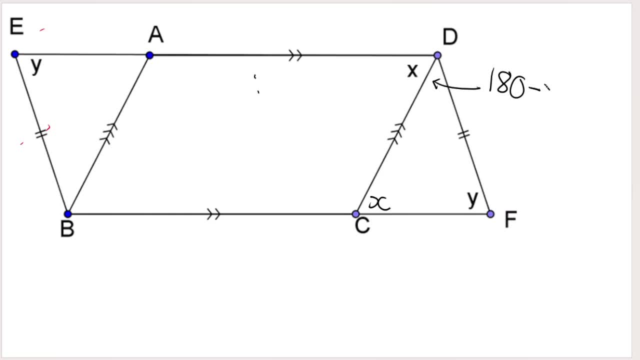 And what I'm going to do is I'm going to add 180.. That angle would be 180 minus X minus Y. That would be this angle over here. What that means is the sum of these two angles over there, to use a different color. 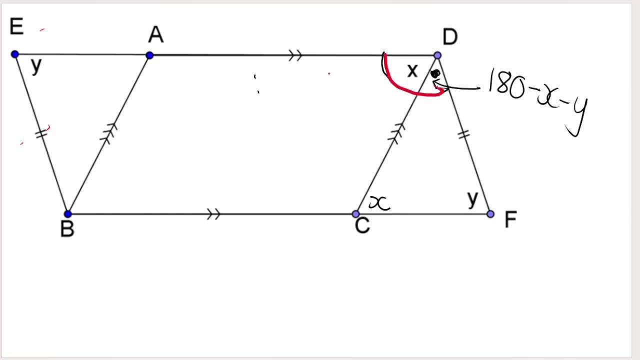 The sum of those two angles Would be X plus 180 minus X minus Y, which is 180 minus Y. So that's this big angle over here. Then the last thing that we did is we added up The angles, The two angles inside the U over here. 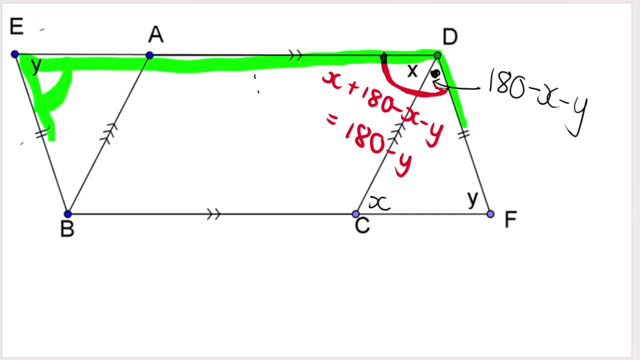 So we added this one, which is Y. So we took Y And we added this big red angle that we just found, 180 minus Y, And that gave me 180.. And because the sum of these two inside angles, these two co-interior angles, equaled or came. 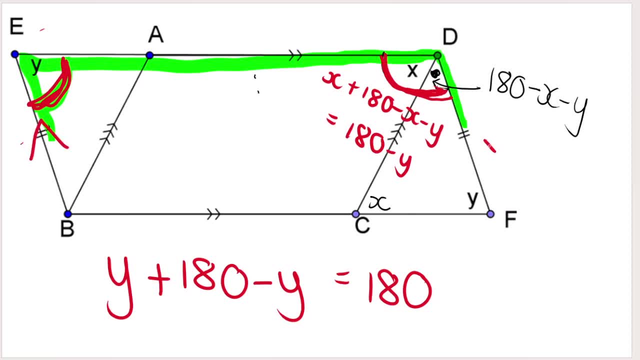 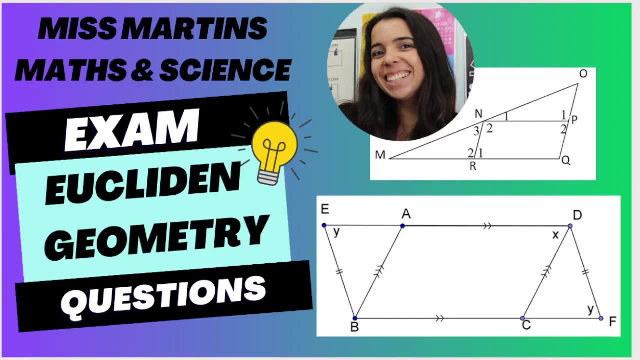 up to 180, we could therefore conclude that these two lines would be parallel. It's the opposite or the converse of co-interior angles. If you liked that video and you'd like to see more Euclidean geometry questions, please let me know in the comments below. I hope to see you for another video. Bye, everyone.